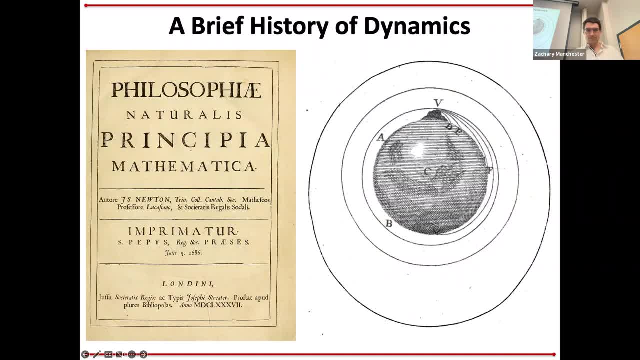 guy. Everyone knows this right. So wait a minute. Sorry, Annoying projector. things are in my way and I can't. Why am I bad at this? I feel like just serious old man vibes here. Okay, Okay, There we go. Okay. So anyone know when the Principia was written? Just for fun. 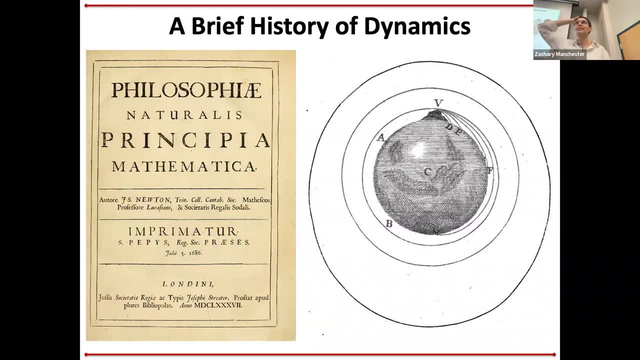 It's like. so it was first published in like 1687 and arguably this was like the foundation of you know all of modern science, basically right Like modern physics, And I mean that's kind of the birthplace of you know physics, analytic geometry, you know calculus, lots of things. 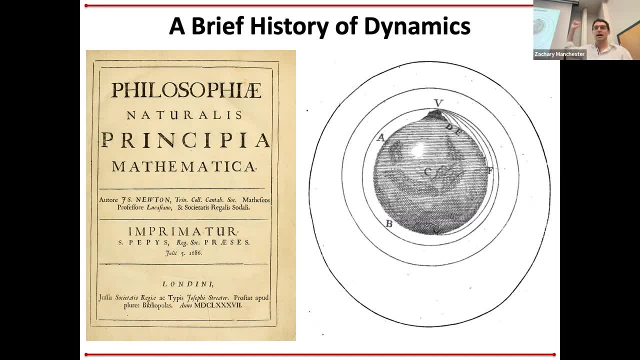 right, And this is where we get F equals MA. It also dealt with gravitation and orbit mechanics back then and pendula and like viscous damping. Basically all this stuff you learned in like freshman mechanics was in this book, you know like 350 years ago, which is kind of awesome, I actually. I think, calculus, there's no calculus. 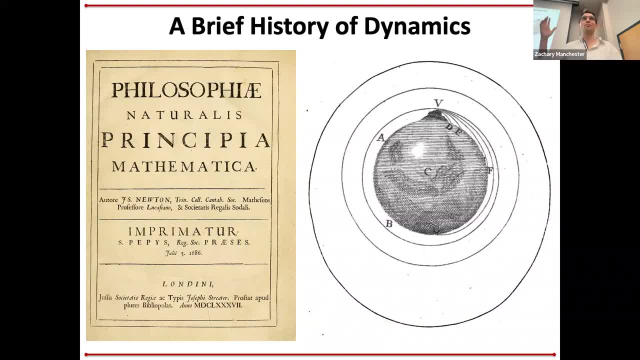 in this book. actually, That's actually wrong. It's all geometric proofs. It's kind of wild and kind of cool And all done with kind of like these kind of vectorial pictures and stuff like that and geometry stuff- Kind of fun. Okay. So what came next? Does this work? Nope, Nope, Nothing works Okay. 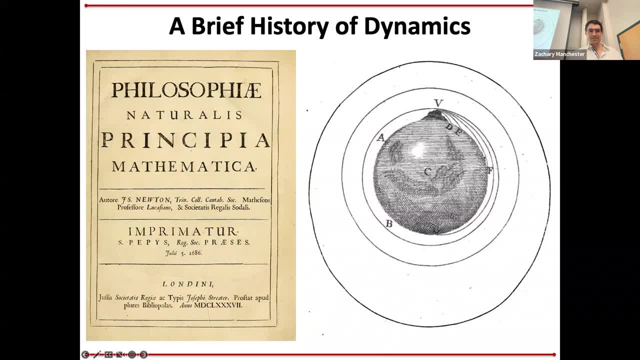 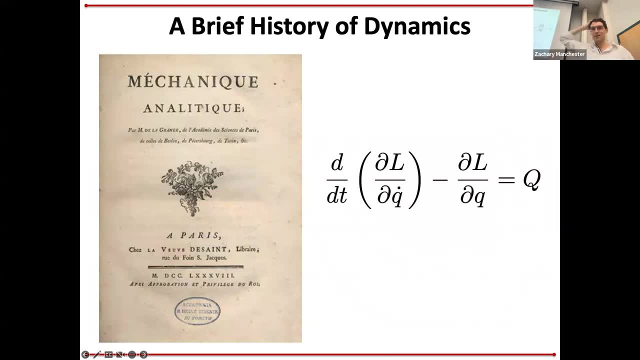 Sorry, I really am striking out today on the. Okay, There we go. So this was the next kind of major chapter in our story. This is Lagrange and a bunch of this stuff. So this was about a hundred years later, a hundred years afternoon. So this is like 1780s, when this was published. 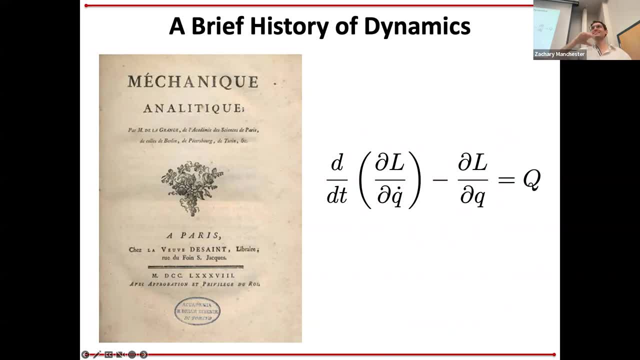 And I don't know what the big story here is. You guys have like read some of this before. So the big deal here is that this book- so whereas the Newton stuff had lots of pictures and was very like draw vectors and stuff like that, Lagrange was sort of super. 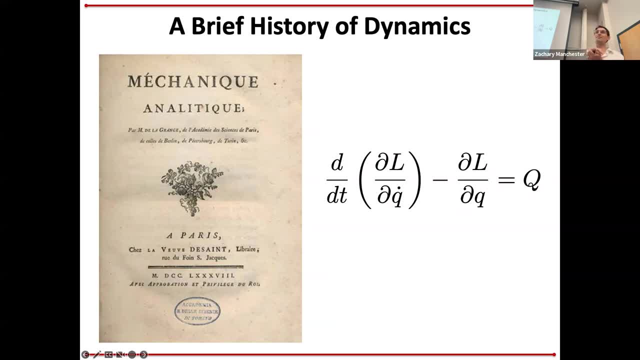 analytic and algebraic and bragged about having no pictures in his book, in fact in like a forward to the book. So this was kind of analytic mechanics, where that kind of thing started. We know that that is. Somebody's got to know what that is. 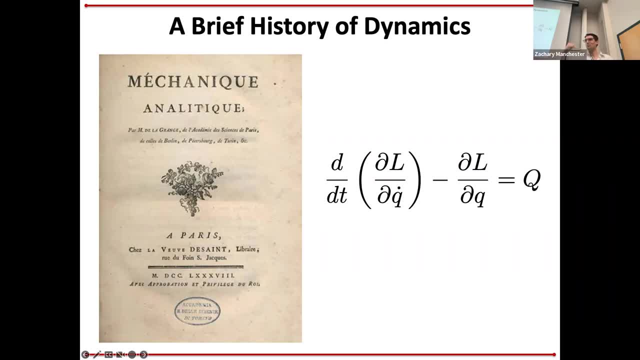 That's the famous Euler Lagrange equation, right? Do you know, like what that is or where that comes from? No, not originally actually. So that's like how you learn it in like a lot of physics classes at the like upper level, undergrad level, And that's completely a historical, like that whole. 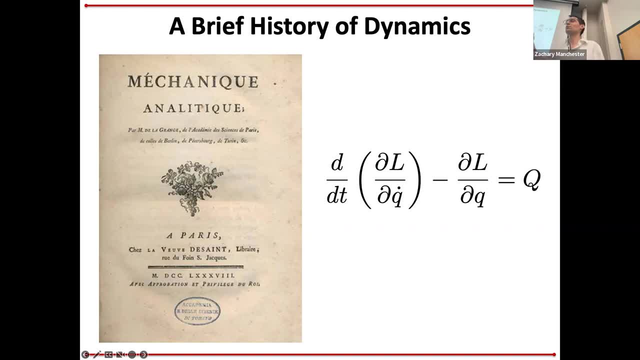 variational thing didn't come to like 100 years after this. So this originally came from taking F equals ma, which is extremely explicitly sort of in cartesian coordinates, and trying to make it coordinate invariant, So basically plugging in like a coordinate transformation. 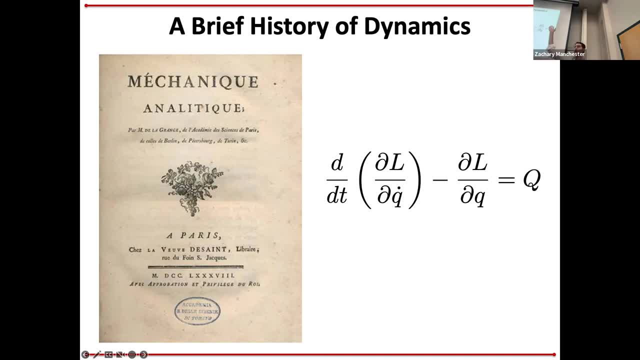 to some arbitrary coordinates cube- that can be whatever you want- And then kind of turning the crank to see what a coordinate invariant version of F equals ma would look like. and that's where. that's where this originally comes from And there are some books that derive it that way, but that's kind of the historical version of this. 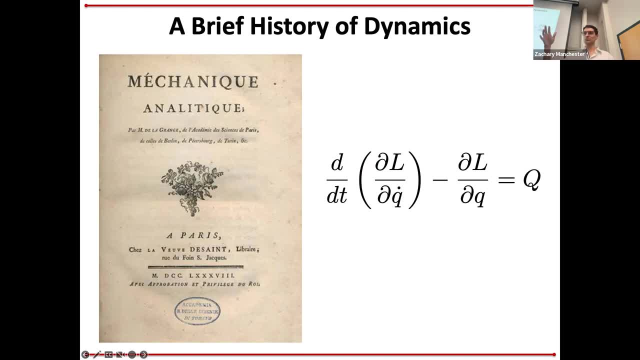 So this was a major advancement over Newton's second law and if it was a ma step, because of this coordinate invariant thing, and we're going to play around with this and you'll see, kind of why this is such a big deal, but this is why you still learn this. 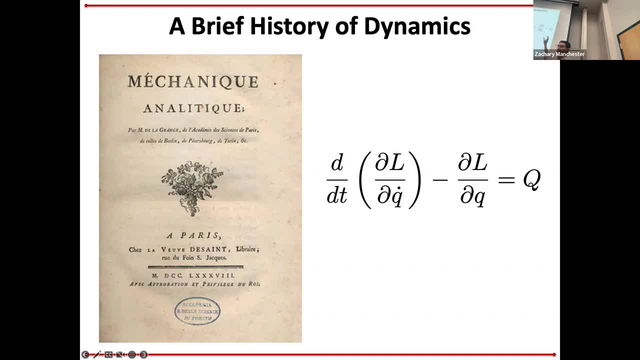 in like sort of senior level mechanics courses and why it's super widely applied in mechanical engineering contexts and and all that stuff. it means that you get to pick your coordinates to be whatever you want, which is super powerful, and it gets us away from drawing little free. 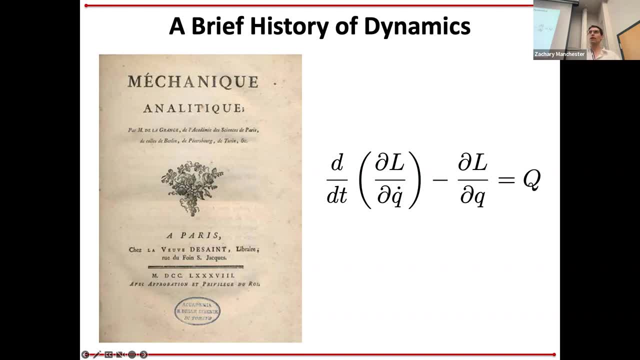 body diagrams of vectors and lets us uh, handle much more complicated uh systems. um, let's see what else is there to say about this. yeah, super practical, we're gonna do a bunch of this stuff- probably a lot of you have seen this- before the next chapter in our story. 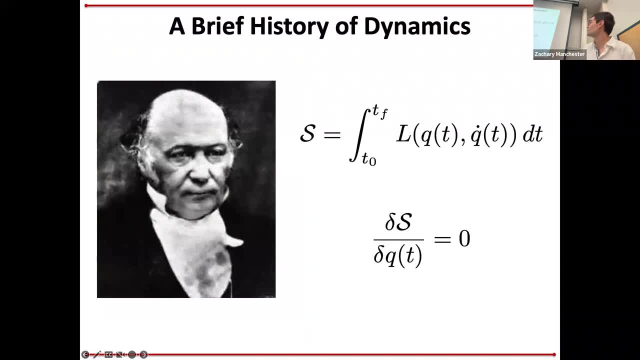 uh, is about another 50 years after lagrange. uh, this is so. it's like 1830s and, uh, they don't know what this guy is, who this guy is and what this is. this is hamilton, famous for two things, uh, both of which we'll talk about in this class. one is this guy. 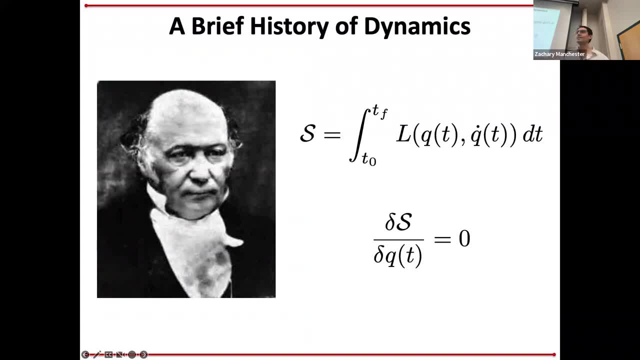 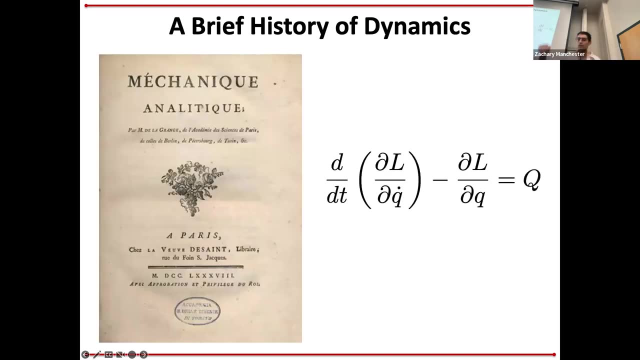 does anyone know what that thing is? that's the action integral. but, yeah, the this thing is actually the least action principle or stationary action principle. so what hamilton did, uh, was take this thing which you know, lagrange, euler, lagrange equation, which originally came from: f equals ma, and this whole coordinate. 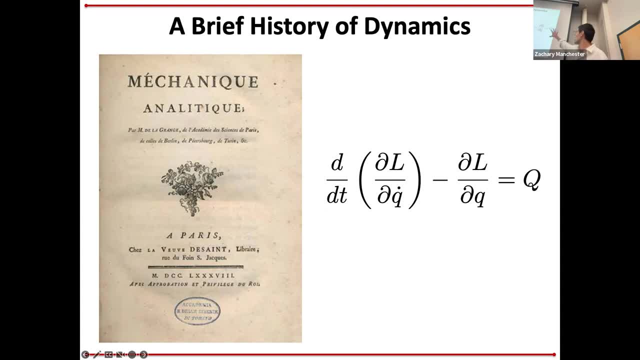 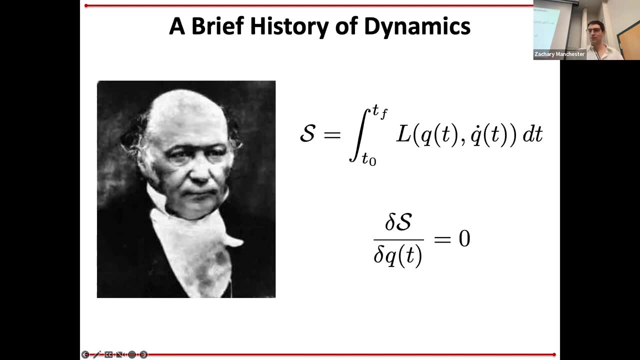 invariance thing that we talked about. basically, what he did was take this equation and really realize this is the lowest action function in the world, uh, and and realize, through some magical intuition or whatever, that, um, this guy, this, the soil of the ground guys, actually the first order, necessary conditions, aka set the gradient equal to zero, uh, for 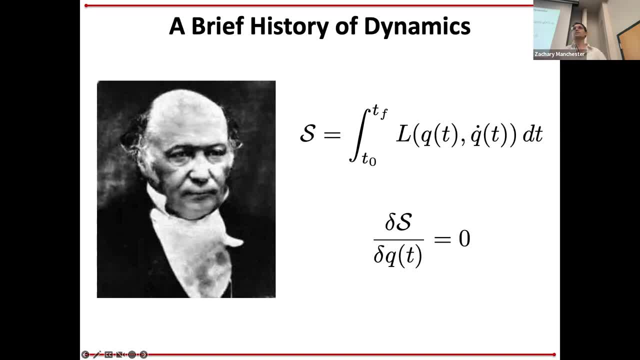 for an optimization problem, which is this least action thing. so if i minimize this thing up here, this s thing, so i treat that as like a cost function, or or loss function, or whatever you want to call it, to the trajectory Q of T. If I do that, the first-order necessary conditions for a local 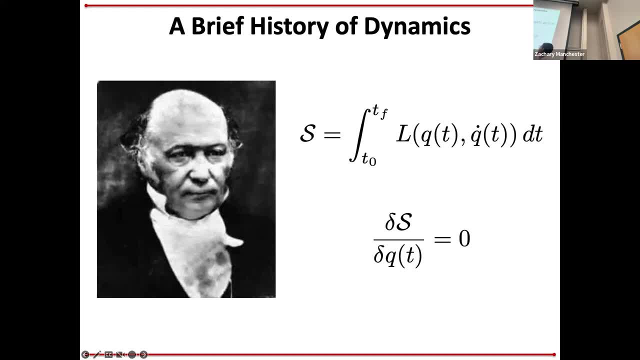 optima is gradient equals zero. That's this guy. If I set that gradient equal to zero turns out opt, pops this guy. So Hamilton's sort of. the big idea from Hamilton here is that we can actually pose dynamics as optimization, And this is cool because it generalizes in a lot of. 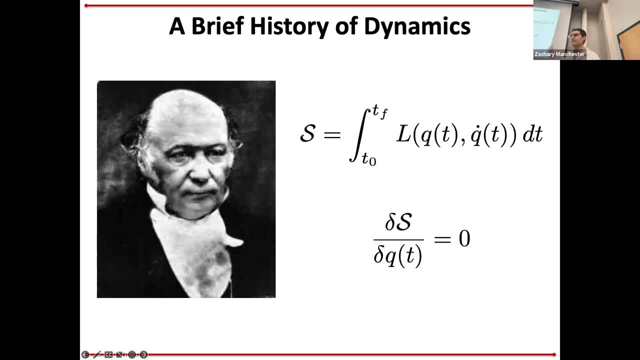 different directions. It lets you now think about adding constraints to this problem in all kinds of ways. We can use other weird coordinates. We can make the velocities and the positions have different coordinates if we want to. We can do all kinds of weird things And it turns out: 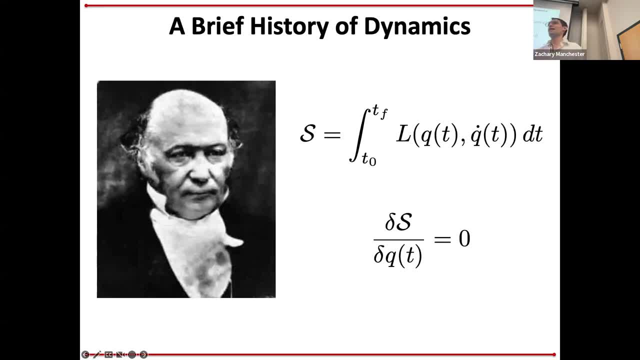 pretty much every formulation of mechanics you've ever heard of passed the Lagrangian thing. So who's heard of some other ones, other ways to get equations of motion, Hamilton Jacobi. Yeah, that's actually. it's a special one that we'll talk about, maybe a little. 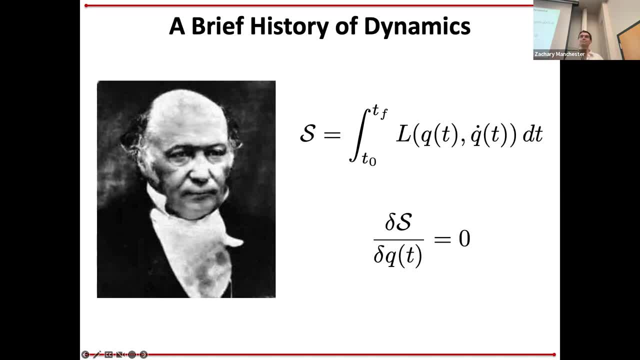 bit Any other ones people have heard of, like the Hamiltonian equations of motion. Have you heard of Keynes equations? or the principle of least constraint? There's all kinds of these things, It turns out. basically all of them are special cases of this guy where you make certain. 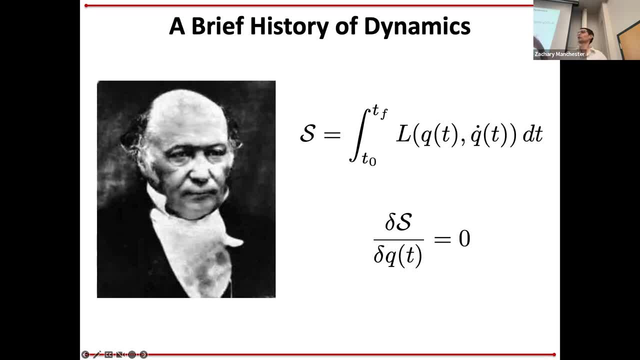 assumptions And you can do all kinds of things. And you can do all kinds of things And you can make certain assumptions about your coordinates or your velocities or whatever, and then turn the crank on setting the gradient equal to zero. So this is kind of the most general setup right here. 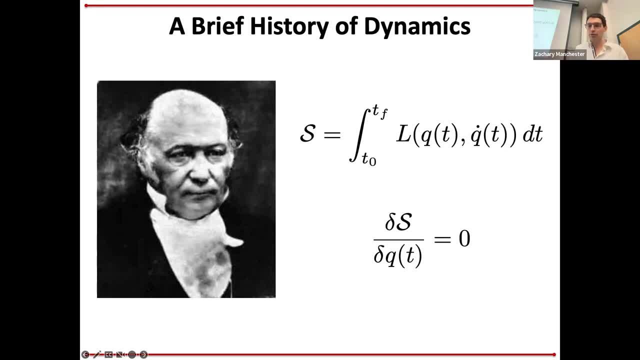 And almost everything else can be derived from this. Super cool. The other thing to say about this is it provides kind of a really interesting bridge between mechanics, dynamics and optimization, right, So we've turned mechanics into an optimization problem, Turns out that's a. 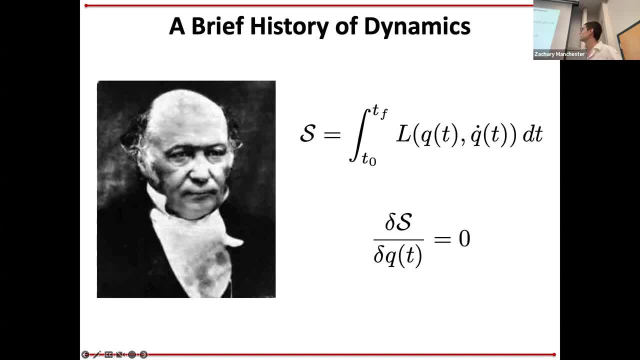 pretty rich vein that you can mine And you can do all kinds of things with it. You can do all kinds of things with it And you can do all kinds of things with it And you can do all kinds of things with it. So 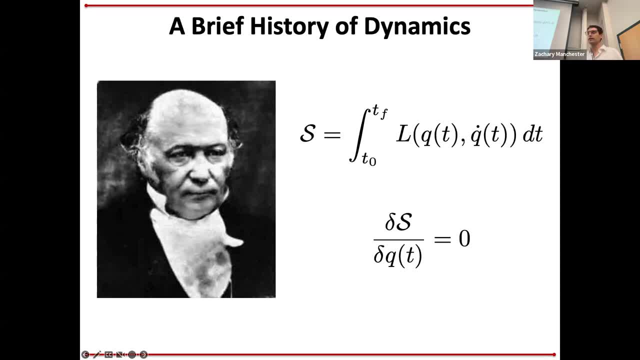 right up to the present day, like in the last 20 years, there's been a lot of work in this sort of direction that exploits kind of deep connections between mechanics and optimal control and lets you derive kind of basically the most state-of-the-art numerical integrators like simulation kind of. 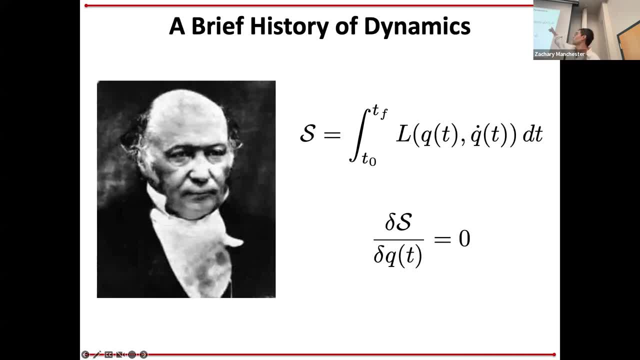 tools for integrating these kind of equations of motion come from this picture and from treating things like optimization problems. Okay, So this is kind of the classic stuff And I'd say this is roughly where classical mechanics ends in physics, But it kept going in engineering. So anyone heard? 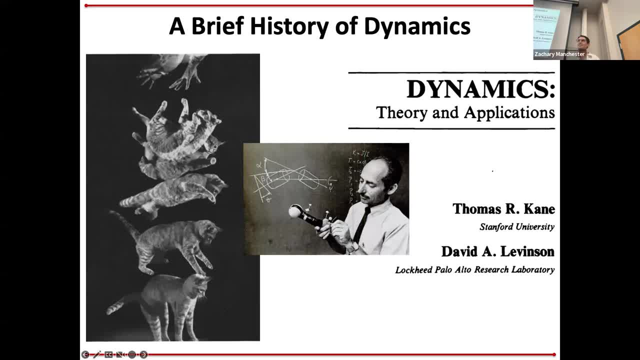 of this guy, Thomas Kane, Kane's equations- Nobody, Okay. So this is kind of fun. Thomas Kane, that's him, I think, he's he, he may, I think only died a couple years ago. So this work was done. 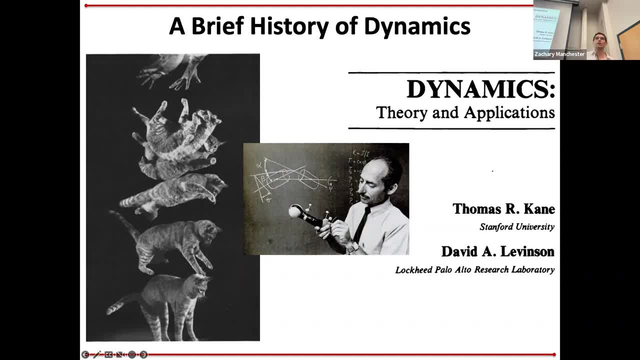 like in the. he was active like in the 50s through 70s. He was a professor at Stanford And he came up with another formulation of classical mechanics called Kane's equations that are actually super popular in in aerospace engineering and have also been widely used in robotics and 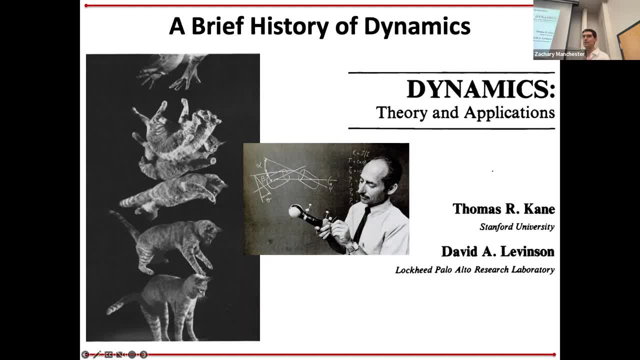 different eras and things like this. He's famous for a couple of things. One is Kane's equations, The other is for actually giving the first definitive solution to the falling cat problem. You ever heard of this? It's super famous, right, Cats always land on their feet. blah, blah, blah. 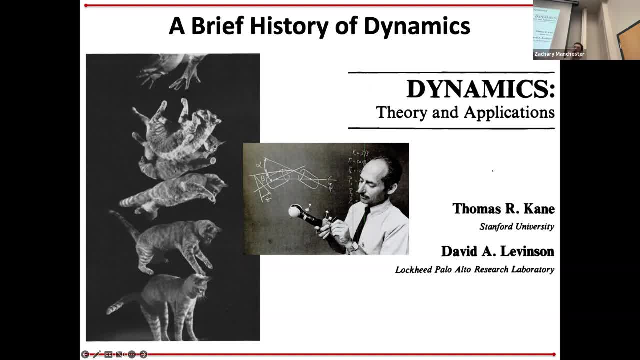 So if you're naive about that, so yeah. by the way, that's a classical, like paradoxical problem, right? So the paradox is: if you have conservation of angular momentum and you have cat dropped upside down, how does the cat flip itself over without like violating conservation of angular momentum? Anyone have? 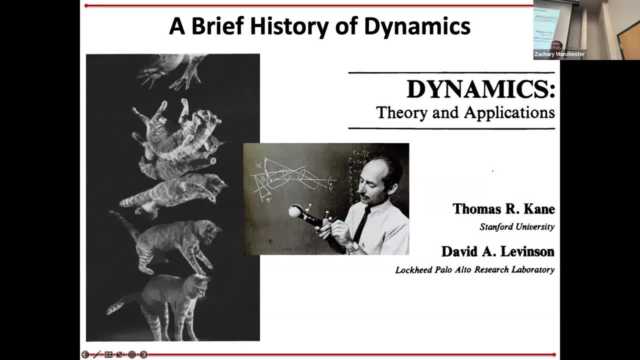 any thoughts. That's the paradox. Anyone know Tail, what Some kind of you know rotates its tail in one direction, you know possibly. So that's kind of the right intuition. Basically the story is the cat is not a rigid body. 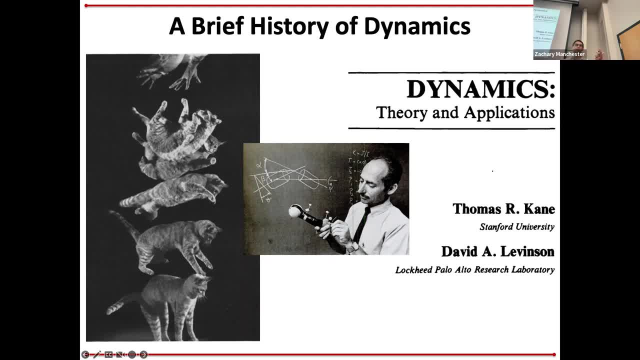 and therefore can manipulate internal degrees of freedom and, like, reorient itself while still conserving angular momentum. So so the tail idea is it's actually not the tail Turns out this is the toy model for the falling cat. It's like a weird dumbbell with a like a universal joint in. 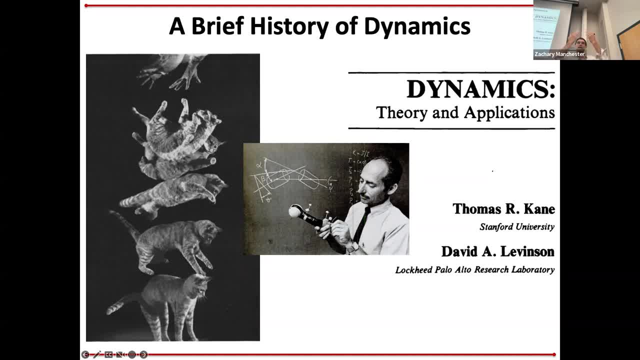 the middle. So it turns out what it's doing is basically arching its back and then rotating its, its spine, And that's what lets it do this maneuver. And so, anyway, that cane actually was the first sort of rigorous mathematical treatment of that like solve the falling cat problem. That 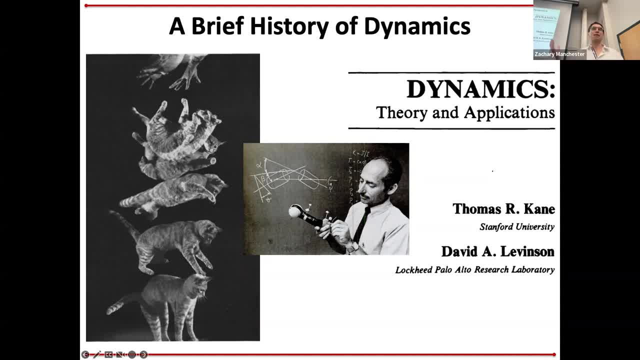 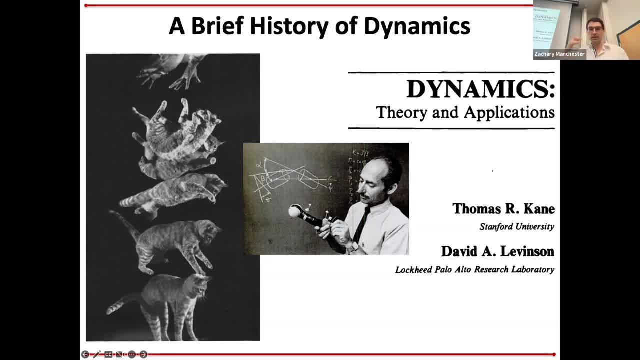 it's kind of sketchy and interesting and fun. So, Thomas Kane, one of the other big things about Kane's equations which we might like touch on, But again they're just a special case of that whole, like Euler-Lagrange, like Hamilton thing, What they do specifically, if you're, if you're. 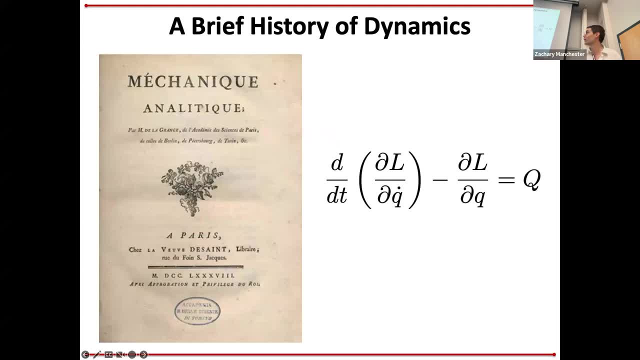 wondering is: in the Euler-Lagrange equation that we we wrote down over here, you pick coordinates Q, but once you've picked your coordinates, your velocity has to be the Q dots right. That turns out not to be convenient in a lot of cases, And in a lot of cases you actually want to have different. 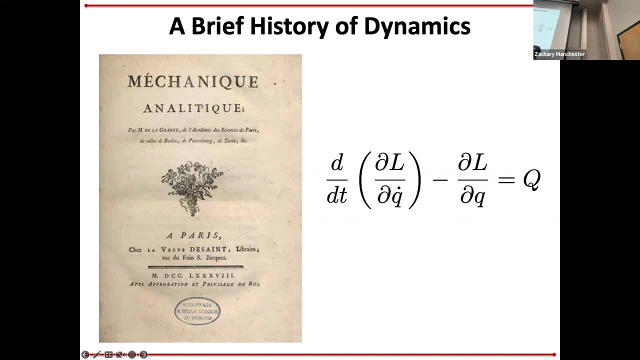 q's. You want to have actually different velocities, v from your q dots. You want to be able to independently choose your velocity variables and your position coordinates and not have to have the v's equal to the q dots. So Kane's equation lets you do that. It basically 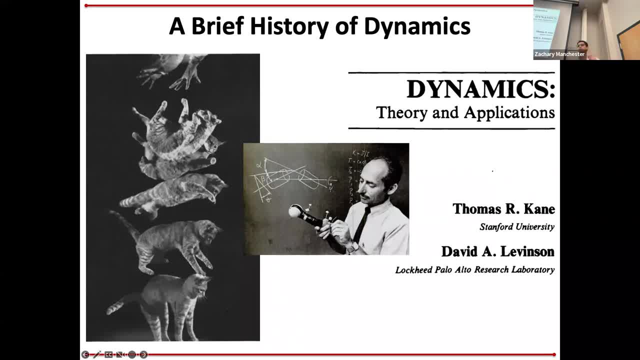 generalizes that Euler-Lagrange equation to have different q's and v's that you can choose independently. One of the fun things about this that's maybe even more famous than the equations themselves is that this work was, like you know, 60s into the 70s, the very dawn of kind of the. 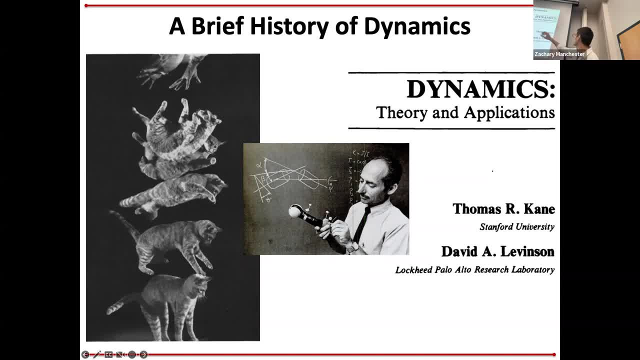 computer age And one of Kane's students, this guy Levinson, who I actually got to meet and hang out with once or twice, developed a software package. that was the first sort of like algorithmic package for like generating equations of motion and solving you know, dynamics problems, like automatically. It's. 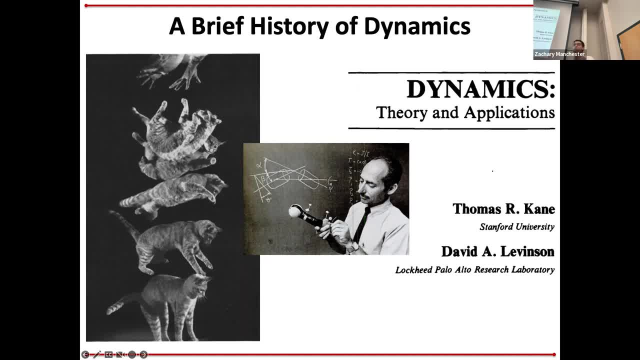 called AutoLev And it's still used in industry And, like now, there's a company that kind of spun it off into another product called MotionGenesis. if anyone's seen this or come across it in internships or whatever, It's still around, And so one of the big things there is that these were 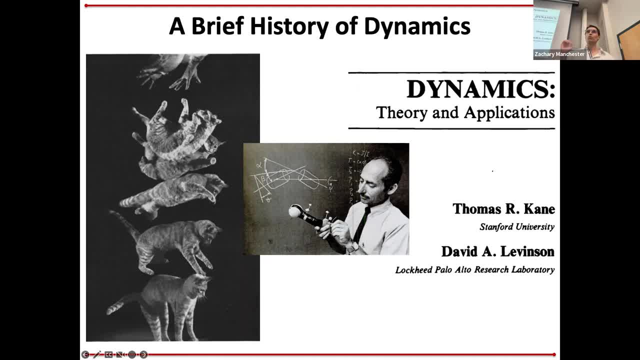 the. this was the first like. these guys are basically the first people to like really try doing this stuff in a computer In a serious way and focus on computational efficiency and like simulation and like formulating of equations of motion. So these guys were the first ones to kind of bring 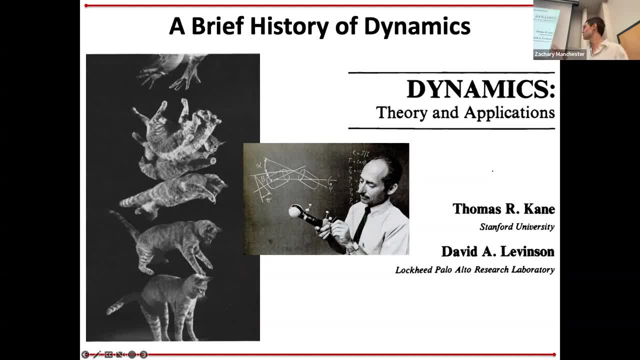 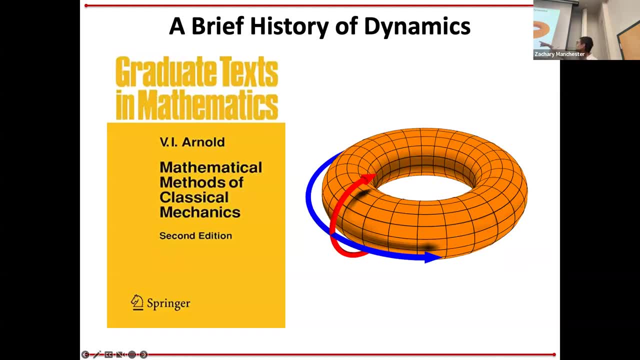 dynamics into the computer age, which is kind of cool, And there's a whole other thread there that continues Some other stuff. we'll talk about this, maybe a little bit. No one's seen this guy before. This book is terrifying. This is the famous Arnold book. Yeah, so you've checked this out. 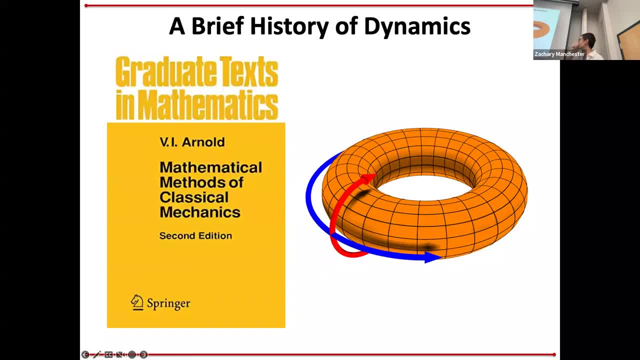 Yeah And yeah. so this book is sort of the most classic book on what's kind of called geometric mechanics and kind of treats. it's a. it uses tools from differential geometry to sort of attack classical mechanics and is probably still one of the most mathematically sophisticated books on. 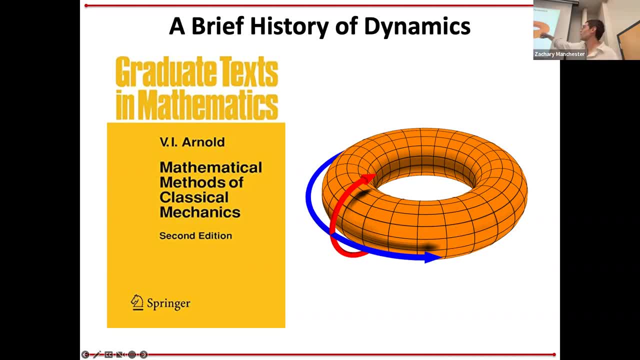 classical mechanics out there. So Arnold kind of kicked this off. He's. he's famous for this thing called the KAM theorem: Kolmogorov, Arnold and Moser- who's another one of these guys in the 60s that has to do with like chaos and perturbation theory. 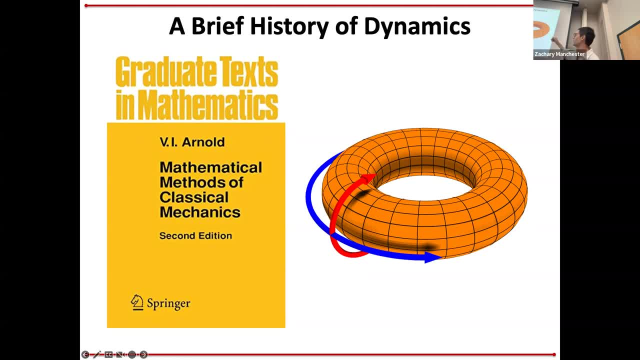 and stuff like this. But yeah, kind of this, stuff's super cool and super pretty and basically, like I don't know what this thing is. It's a torus, a two torus. So it turns out that is the configuration space for a double pendulum. 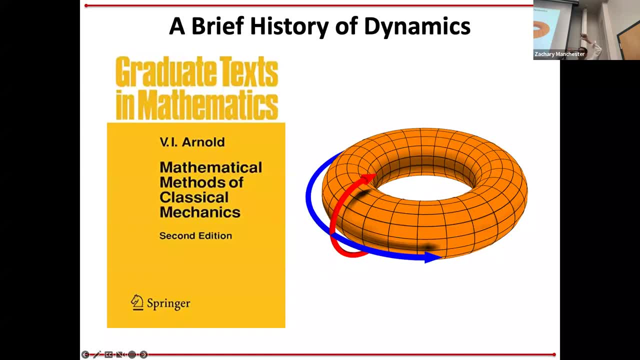 Yeah, So a double pendulum has two angles, a theta one and a theta two. Hopologically that's a torus, right, You've got theta one, say, in blue and theta two in red. So if you think like geometrically that's, that's actually the space, that the dynamics of a 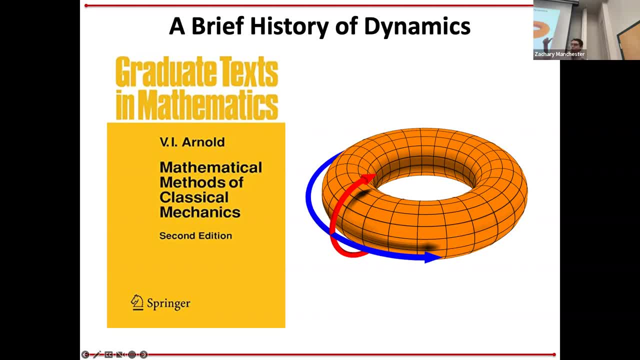 double pendulum evolves on. So this is kind of the perspective It turns out by, like looking at things like from this perspective, this geometric perspective, right, there's a lot of cool things you can do There's. there's really beautiful theories that you can do There's. there's. 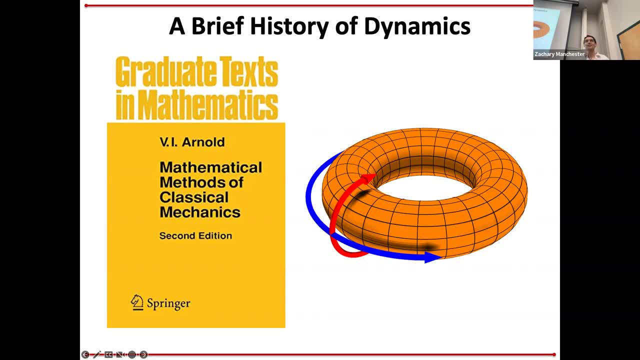 really beautiful theory, but the math is like pretty rough and the notation is particularly rough. So we might we'll, we'll, dabble in this stuff a little bit, but we're not going to like go to too crazy. But yeah, the big thing here is that what these tools can do for you is kind of 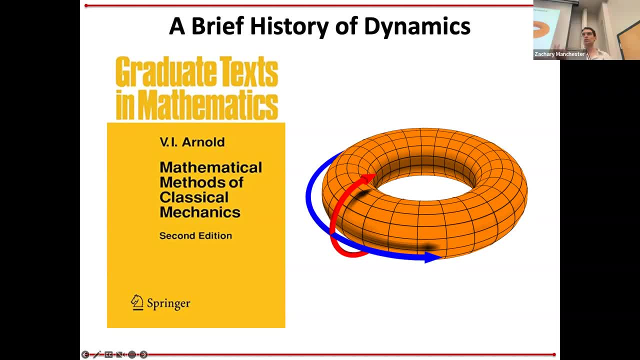 provide a lot of insight into the kind of like structure of the solutions to these equations, even in cases where you can't solve the ODEs explicitly right, So you can't get a closed form solution. You might be numerically integrating them in a computer, but 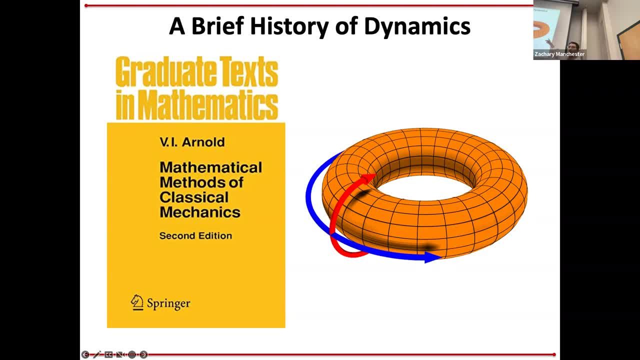 but there's still a bunch of structure in there, right, A lot of geometry kind of stuff like this and this can give you insights into, like conserved quantities, right, Conservation laws, symmetries of the system, things like that. that can help you sort of think about the dynamics in qualitative 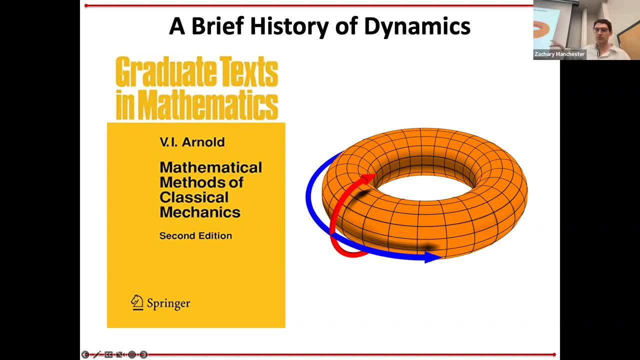 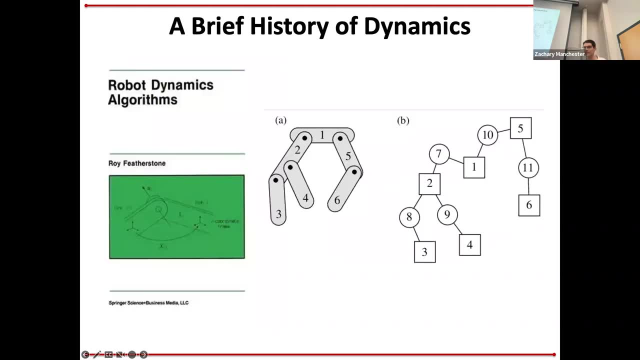 ways that are kind of interesting. Okay, so that's sort of geometric mechanics. This is 20th century stuff: 60s, 70s, 80s. Another thread coming from computer science: Anyone heard of this guy? Featherstone? Okay, so, yes, a couple people, No. okay, so Roy Featherstone, This is like 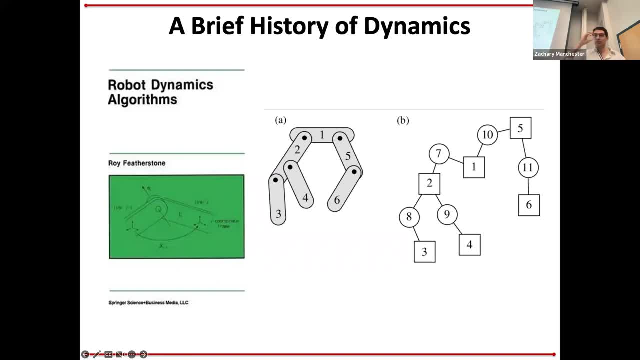 late 80s- He's still around, still doing it- He developed the first general linear time algorithms for dynamics. So what kind of idea here is- and this is coming from robotics now- so the idea here is, if you have like a robot arm, this thing is what we'd call an open 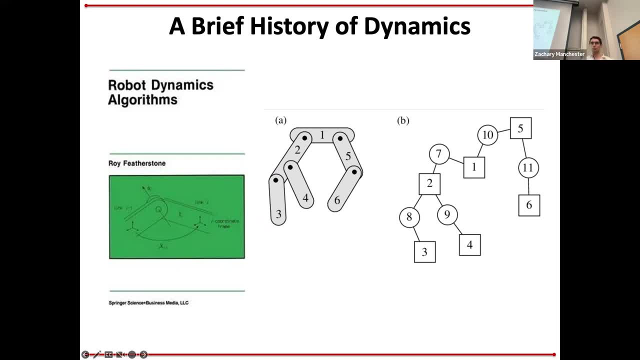 kinematic chain, So there's no loops. It turns out that there's a bunch of sort of topology and graph structure there that you can exploit in order to solve the equations of motion. So if you're going to like simulate a system in linear time in the number of degrees of freedom, 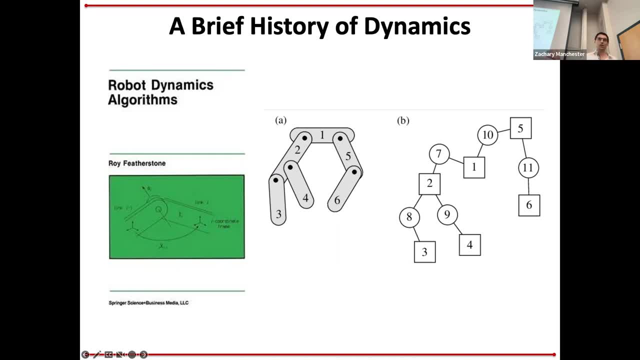 it turns out, you can do that in general for an open kinematic chain, So anything that doesn't have loops, which is humans. you know quadrupeds most, you know robot arms, things like this, Which is pretty cool, It turns out. does anyone know what the complexity is if you don't do this? 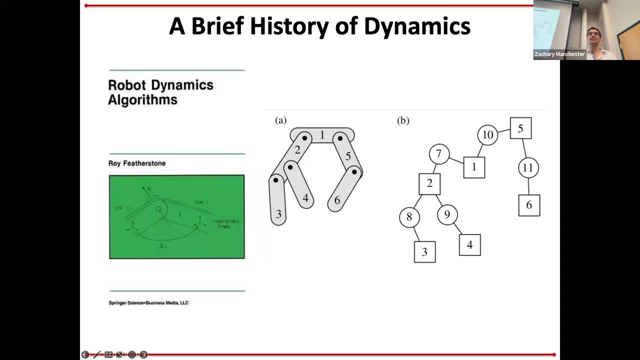 clever stuff. It's actually fun. It's actually easy to show this, but does anyone know offhand, It's cubic. So if you can go from cubic to linear for a big system, right, if you have like a humanoid robot with, like you know, 40,, 50,, 80 degrees of freedom, that's you. 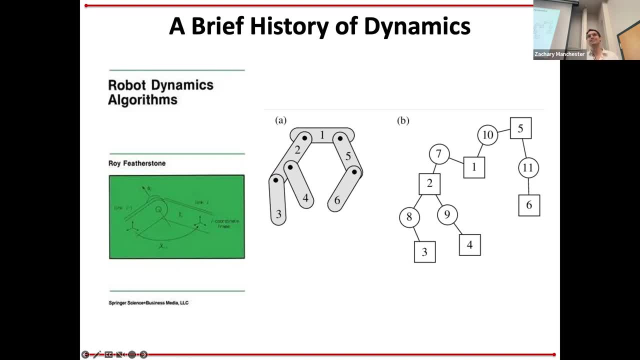 know 80 is much smaller than 80 cubed right, So it's a big win. Does anyone know where that cubic complexity comes from? It's a fun one. So in order to get like q, double dot or velocity. 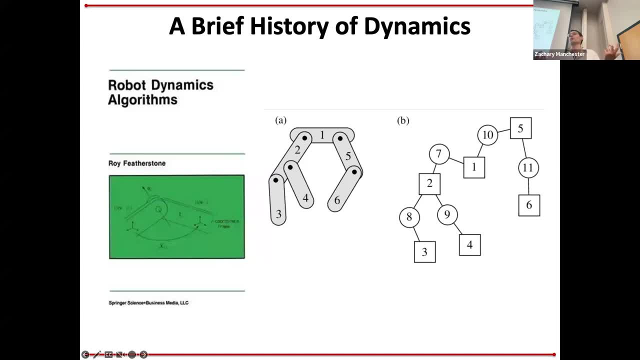 you know accelerations out of equations of motion. you have to invert the mass matrix and that's n by n in the state dimension. And inverting a matrix or solving a linear system is cubic in n right. So if you just write down, you know Euler-Lagrange stuff. 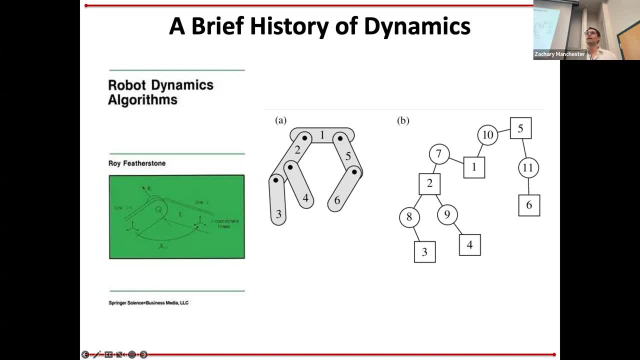 you get a mass matrix. It's cubic because you have to invert that thing And basically by being super clever with, like you know, tree structure and stuff like this, it turns out you can. you can basically solve that linear system effectively or factorize that matrix in linear time, which is cool. 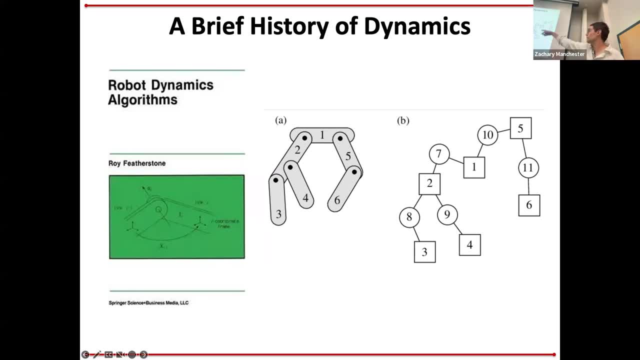 What else is there to say about this? So okay, so Featherstone, that book. there's a newer edition of this too. that's pretty recent. last couple of years Did that in what are called minimal coordinates or joint coordinates or generalized coordinates. 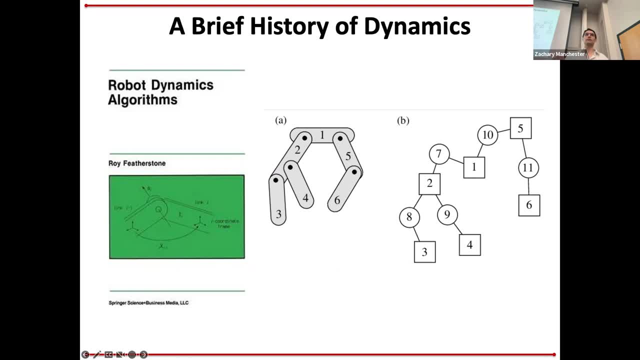 And then in the 90s a guy named David Barath, who was a professor here in RI, showed how to do this in linear time in so-called maximal coordinates, where you basically write down the full sort of coordinate representation for every link in the robot. 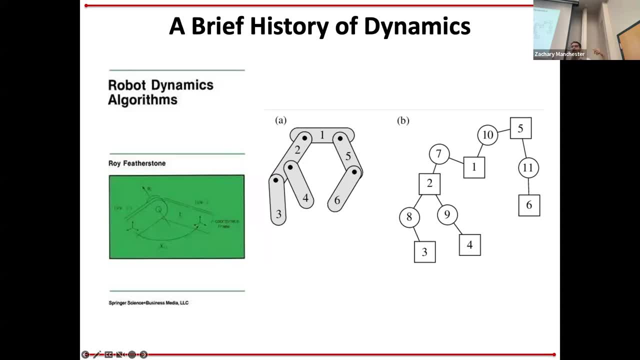 and then write down explicit joint constraints with Lagrange multipliers, So he showed how to do linear time stuff in that context- sort of early 90s- And the whole story behind this, though, is sort of exploiting this kind of graph structure stuff in the system. 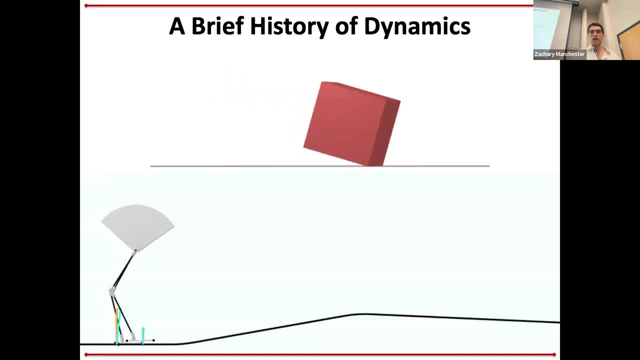 That's kind of the idea. Okay, so that stuff, what else is there to talk about? Okay, another line of work. that's sort of again from the robotics side of things. it turns out in robotics we care a lot about this kind of stuff. 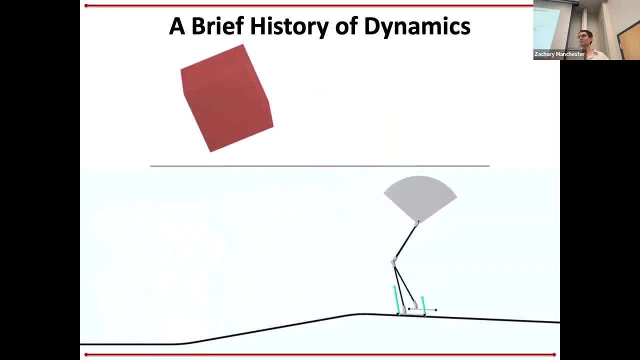 impacts and friction. Has anyone ever tried writing down or simulating systems with impacts and friction, like walking or grasping, or yeah, a little bit? So if we're being super rigorous, we're thinking rigid bodies. what happens to my velocity when I do this? 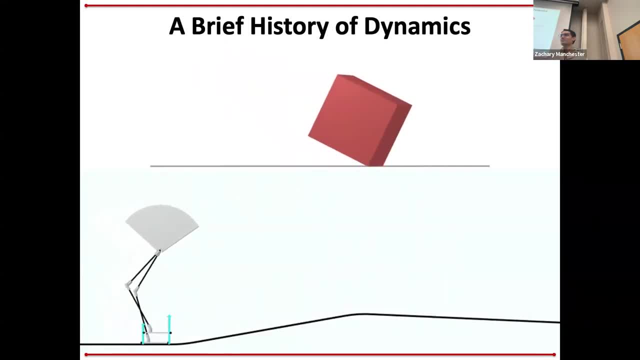 It's a rigid body. Yeah, it instantaneously goes from whatever at like T plus epsilon to like zero when it hits under the rigid body assumption which is idealized, and blah blah blah. but that's a pretty good approximation to most things in robotics, right. 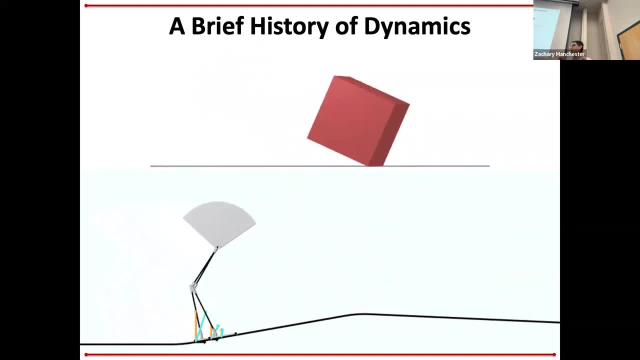 So it turns out, strictly speaking, with that velocity, discontinuity, what are my accelerations? And if I try to write that down with F equals MA, falling brick, falling brick, what happens at the instant of impact to F equals MA? 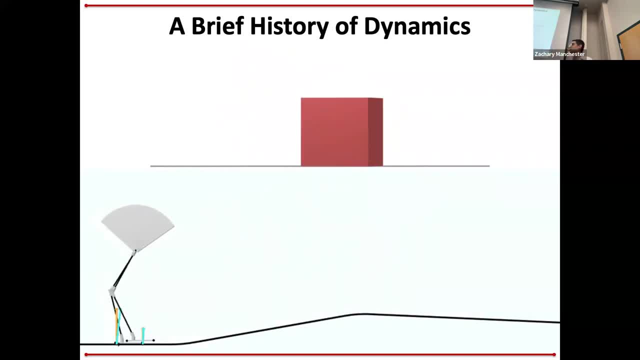 Yeah, so it turns out rigorously speaking, you can't do F equals MA. here It doesn't work right. You get like infinite spiky things. If you want to be mathematically rigorous about it, you have to think about these things. 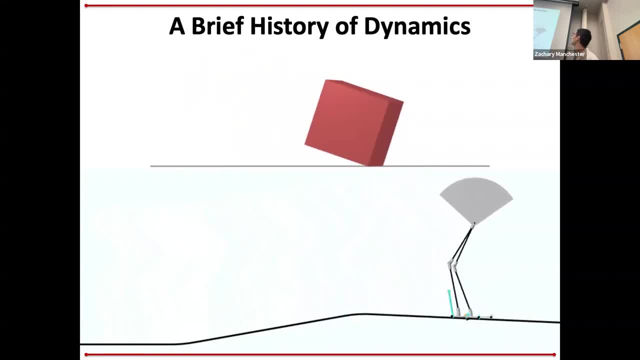 called measured differential inclusions, and we don't want to do that, so we're not going to go there. But basically this gets really weird and there's a lot of pretty gnarly math if you want to treat it rigorously. 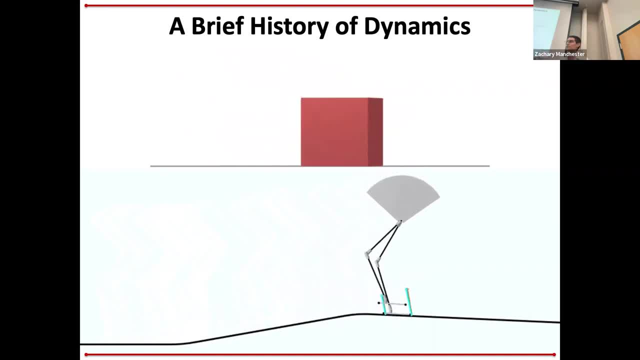 and you can't quite apply vanilla F equals MA to these things. So you have to think about these things as like assuming idealized rigid bodies. What actually happens in reality is that these things all deform a little bit and there's a little compliance. 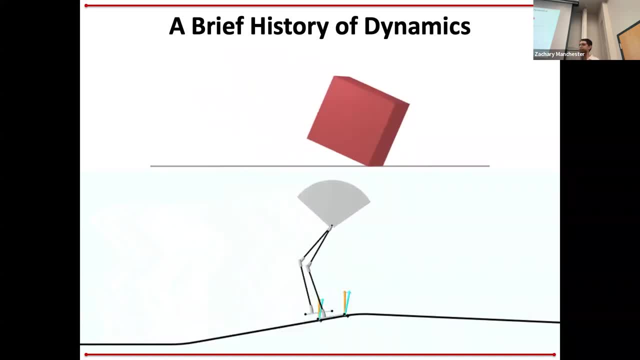 and a little give and internal degrees of freedom and whatever that's dissipating energy into vibration modes and bending modes and the objects and stuff like that. But to do that you have to resolve these really fast, really fine scale dynamics in the objects. 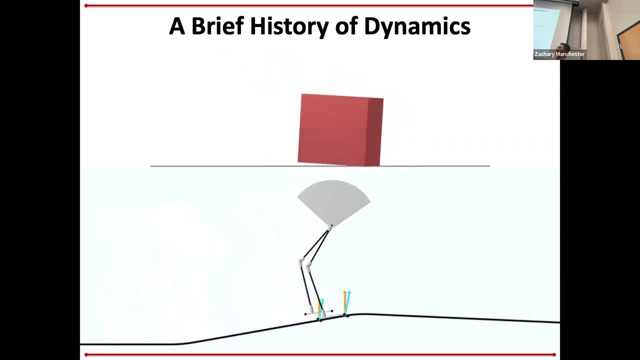 and we don't do that, We don't want to do that, We don't want to have to think about the- you know, I don't know- Vibration modes of the feet in my robot that are tens of kilohertz or whatever. in order, 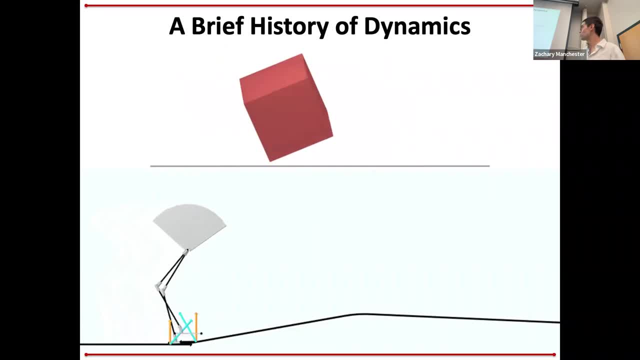 to simulate walking, and we don't. So it turns out that the rigid body assumptions are still pretty good here, but a lot of weird things happen. So the first really mathematically rigorous treatment of this stuff happened in the 1970s. 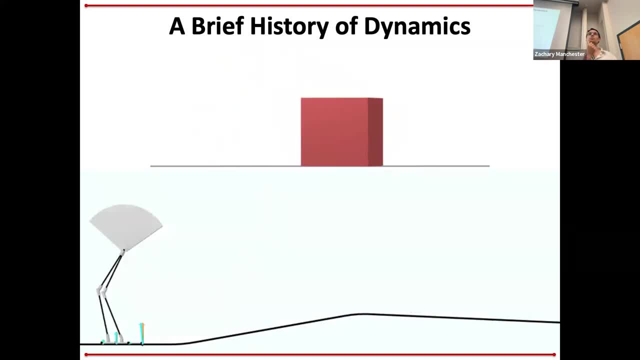 by a French guy named Moreau, and he developed this thing called the maximum dissipation principle, which is the sort of rigorous analytic variational theory that lets you describe stuff like this And surprise, surprise, it's an optimization problem. We'll talk about that. 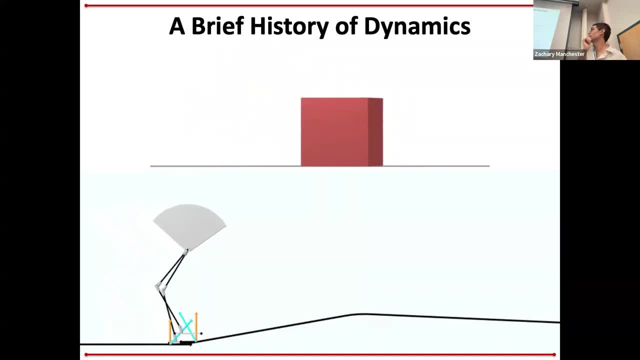 And then in the 90s the first actually usable general simulation tools for stuff like this came out. The seminal paper is Stuart and Shrinkel, which is like 1997 or 8.. And then there was a follow up one in 2000. 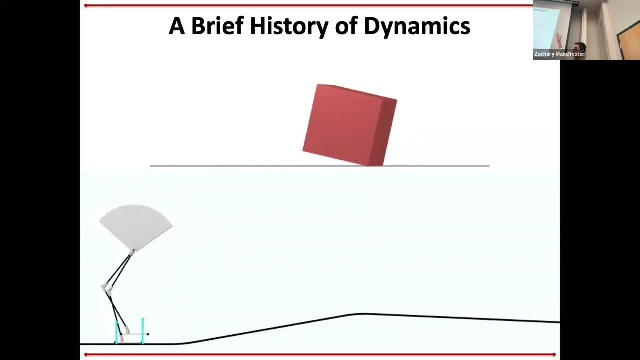 that kind of fixed some bugs in the original paper. So really we're talking like the first stuff to do this rigorously wasn't until like 20 years ago, right, Like It's kind of interesting, And these are called time stepping methods, which 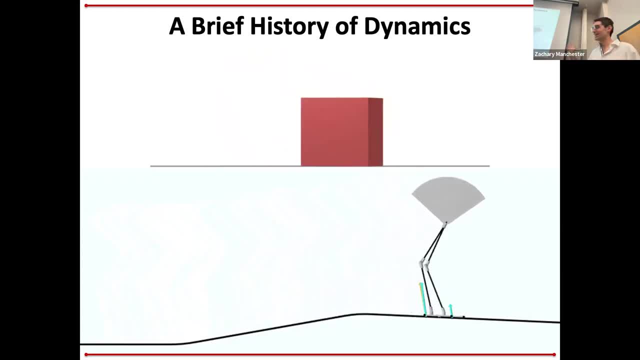 is kind of ambiguous and not very descriptive, but that's what they're called. What else is there to say about that? And that's actually what's underlying a lot of current robotics, particularly bullet- if you guys are familiar with PyBullet or whatever that. 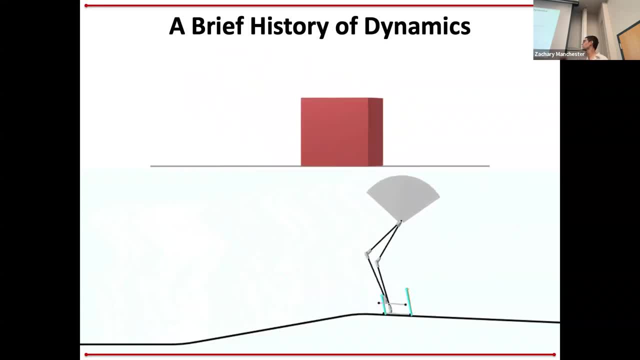 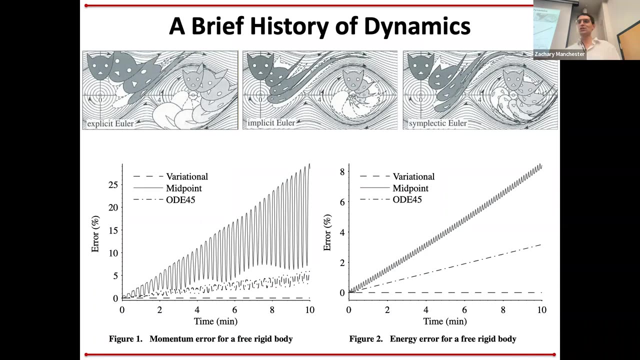 uses Dart also does this time stepping stuff of Stuart and Shrinkel fame. OK, what else is there to say about things? OK, Other fun and weird things that we will do in this class. I mentioned the like geometric mechanics stuff. It turns out there's a whole body of work. 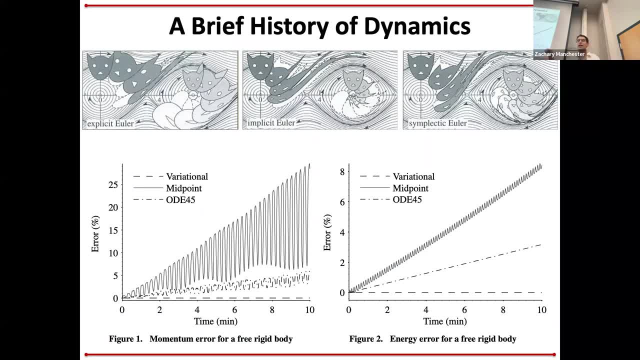 on deriving numerical simulation methods, AKA numerical integration schemes, from those ideas that conserve energy and momentum and all this good stuff. So what you're seeing here is like a sort of standard, say like ODE45 and that type of thing, Compared to like a variational integrator. 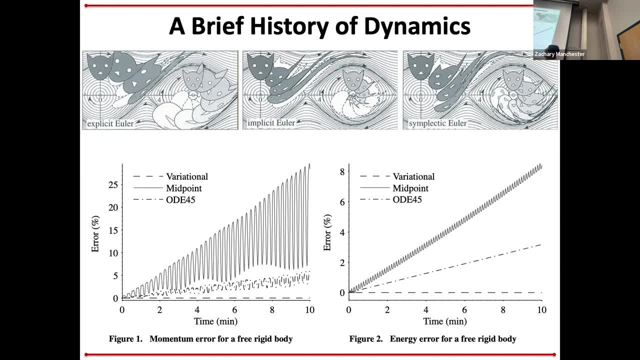 See, there's like tons of drift in the momentum energy, whereas this like variational integrator just is exactly conserved to machine precision, conserving all of the conserved things right. So that kind of comes from that geometric picture. Yeah, that's like a weird phase space illustration. 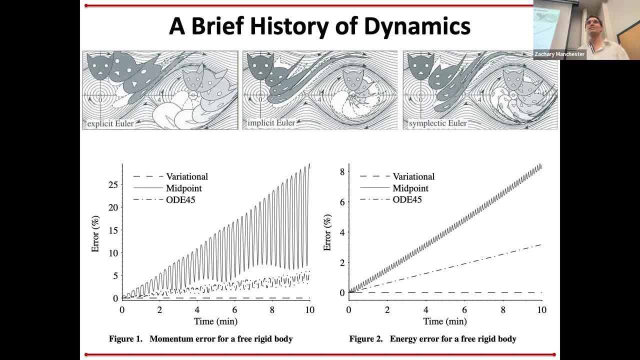 of this on a pendulum on top with a cat face From. the cat face thing actually comes from the Arnold book, OK, And it became kind of like a meme in mechanics books ever since. So I think this particular cat face thing is not from the Arnold book. 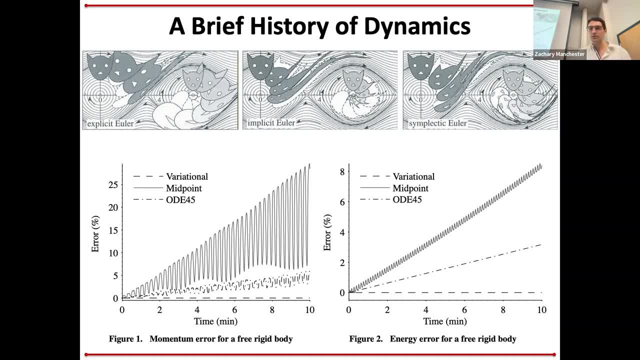 They stole the cat meme from the Arnold book, Anyway. so yeah, we're going to go kind of deep on this, on these like structure preserving, numerical integration methods, because I'm into them. I think they're super cool and useful, But they're not widely used, which I think is a bummer. 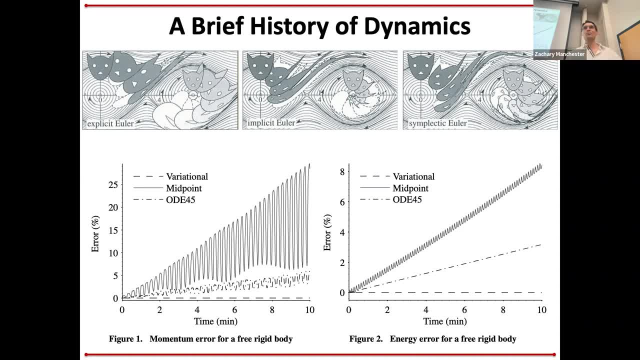 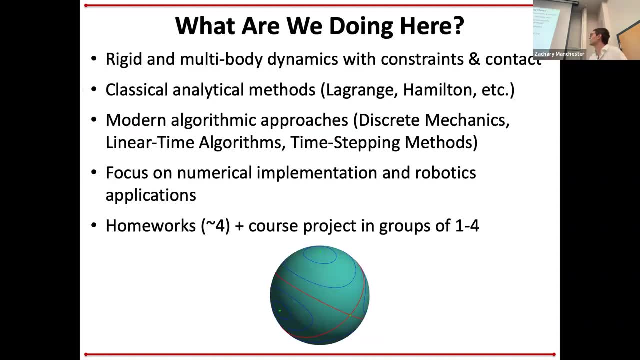 So maybe you guys will fix that, OK. so this is my weirdo whirlwind tour of mechanics topics that we're going to cover And, one way or another, some more logistical things, So high level what we're going to do. 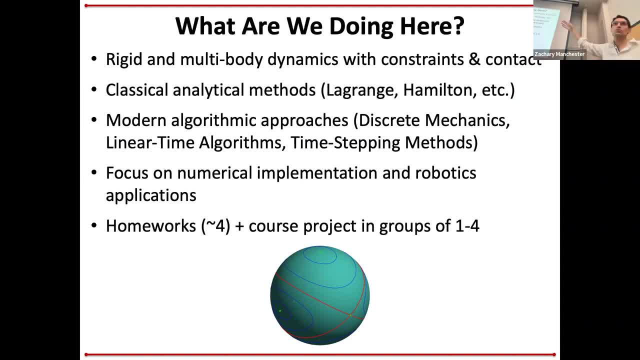 a bunch of sort of rigid and multi-body dynamics things. Particularly we're going to cover constraints and compact. So all that impact friction stuff that happens in robotics that's super gnarly and weird and hard to simulate. we're going to do it the right way so that you guys don't have 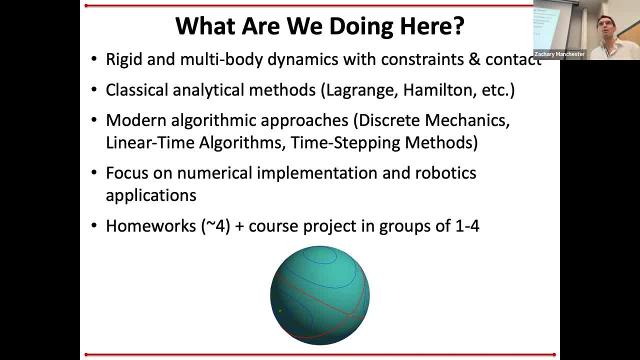 to use hacky MuJoCo things or spring damper models or whatever that are terrible. OK, We'll do kind of the classical analytic stuff, so like the Lagrangian, Hamiltonian stuff, And then we'll take a tour through kind of a bunch of like kind of modern or state. 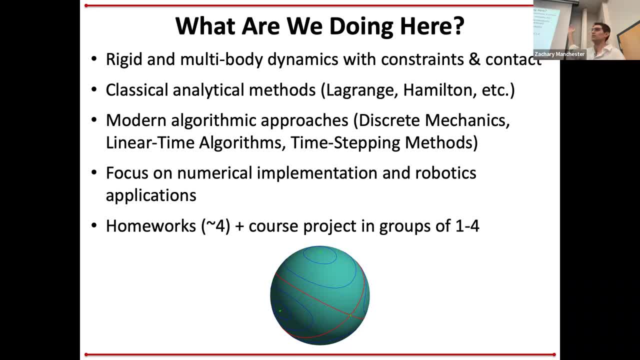 of the art algorithmic ideas. So these discrete mechanics things, these structure preserving integrators, the linear time algorithms, the Featherstone stuff I mentioned, and these time stepping methods for simulating contact. So basically, you will have the tools to build your own state of the art simulation of whatever. 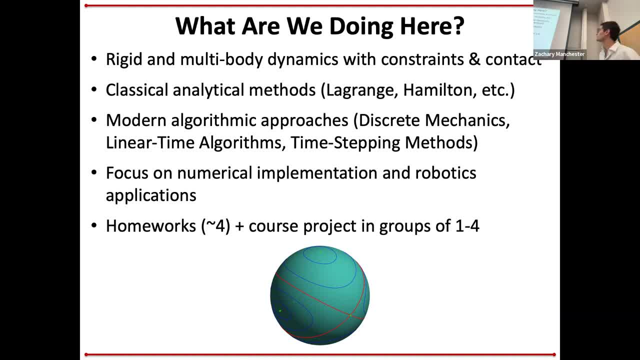 thing you care about, like whatever robotic system you care about. That's kind of the idea. And again, yeah, like a lot of focus on numerical methods. implementation We're going to the homeworks will be code based, like implement algorithms and try stuff out and like stuff. 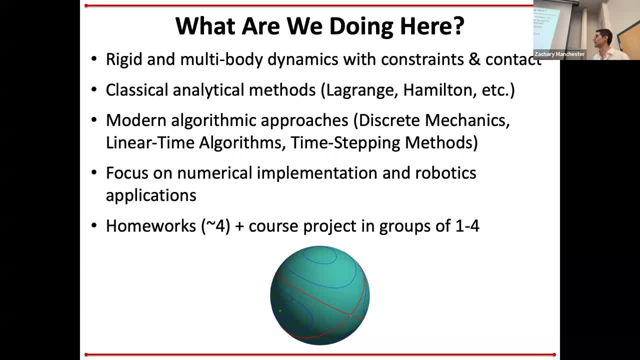 that's heavily biased towards robotics applications. So we'll do a lot of case studies with, like drones and arms and legged robots and all this kind of stuff, which, hopefully, is what we're all into here. OK, So yeah, There'll be like four homeworks. 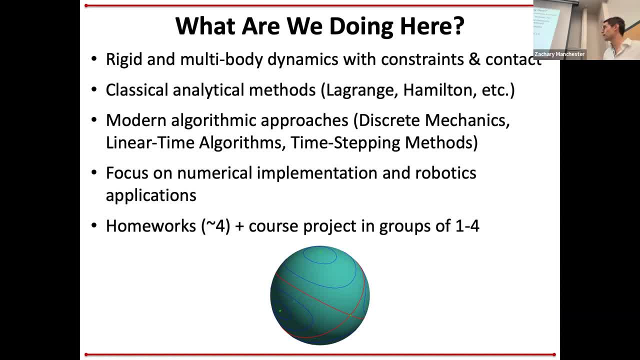 And there won't be a final exam or anything. We're going to do a course project And the idea there is: you can do it in group, You can do it by yourself, Kind of up to you. I said up to four. 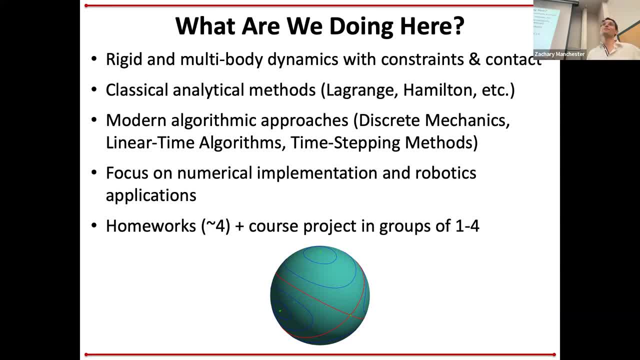 There's no, that's an arbitrary cutoff. If you have five friends and you really want to work together, we can do that. That's fine, Come talk to me. The idea, though, is to- basically- it's super open ended- Do a project on something that you 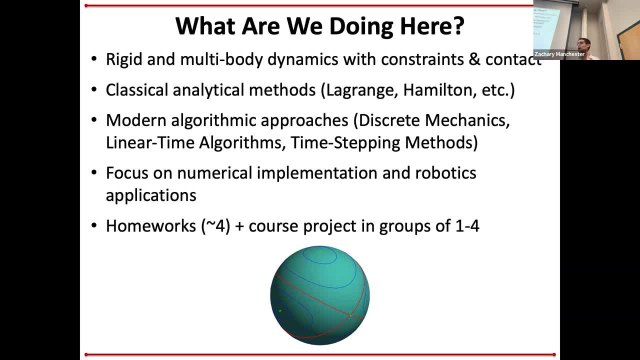 think is cool using stuff from class. That is it. So the intention is it's a graduate course And what I hope is that you guys are sort of doing research where these ideas and stuff we're going to talk about here is useful for you. 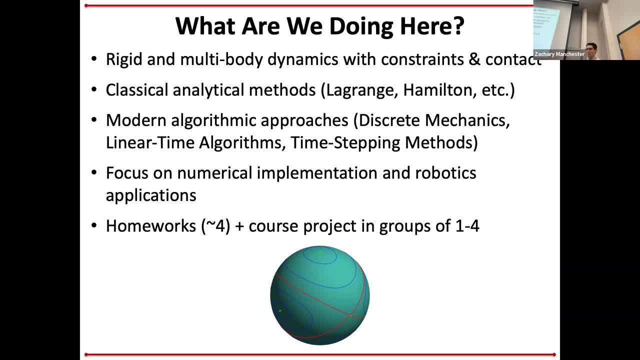 and your research. So the idea is not to make you do more work or whatever. The idea is for you to get something out of this class and use the stuff in your own research. So the hope is that you can kind of spin a conference paper out. 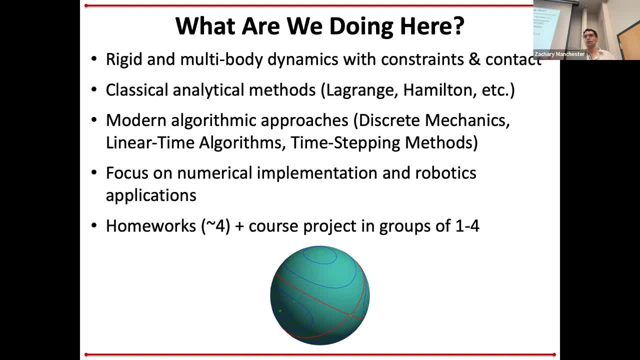 of this. So do something cool and relevant to you that you think is interesting and hopefully it'll overlaps with your research. You'll write it up for the class project and hopefully you can kind of take that and go submit it to something. Any questions about any of this stuff? 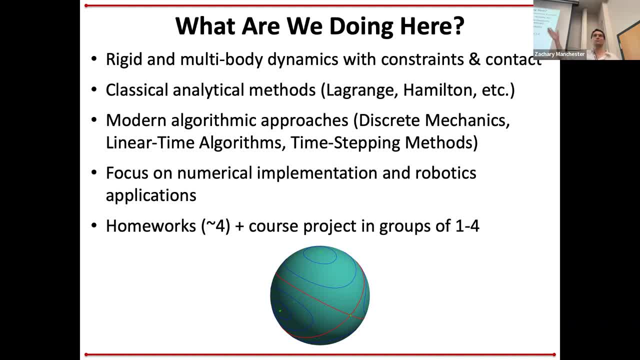 It's kind of the gist of it: Almost every two weeks and then the end they'll sort of stop giving you homework so you can work on the project towards the end. I think that's kind of it. Any questions about topics, this stuff, all good. 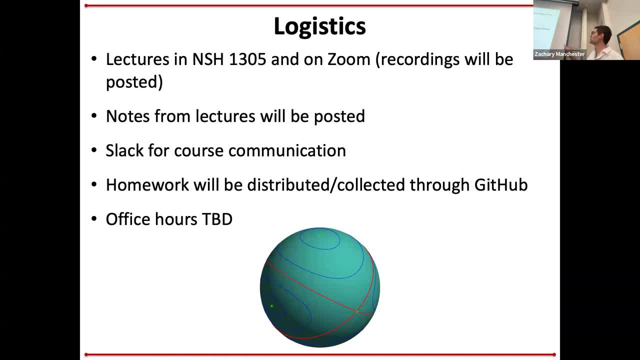 OK, and then, I think, the last logistic stuff. you found the room, so that's good. I'm also going to live stream it on Zoom, because I've been doing it for the last year and a half and it's easy enough, So I figured there's no reason not to. 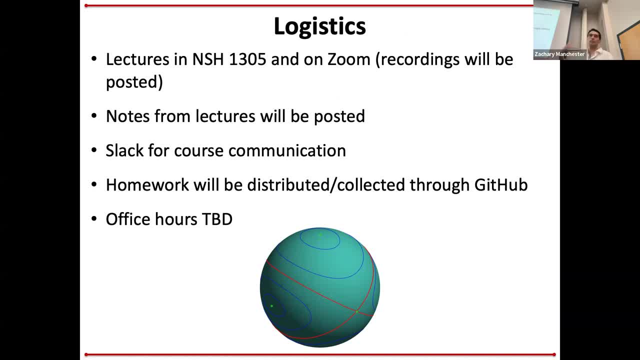 So I'm doing it now, I'll post the links and stuff And I'm also recording them and I'll post them on YouTube So you can go back later or whatever. If you're sick or something, you can watch them there. 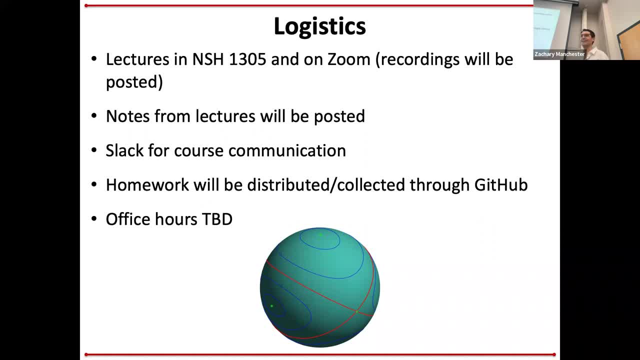 I'm going to write notes on an iPad which I think thankfully got working after much struggle today, So I'll post the notes also online. I like using Slack and kind of hate Canvas and Piazza, So given the course size, I think that's manageable. 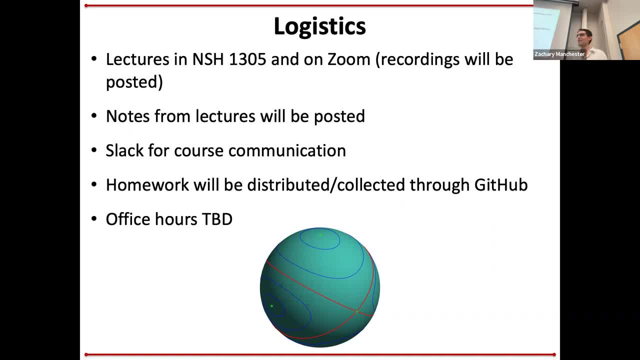 We used Piazza for the last class because it was huge and Slack was unwieldy. But I think there's a manageable size so we'll go back to Slack. So, Slack, you can bug me, you can bug Anthony on there. 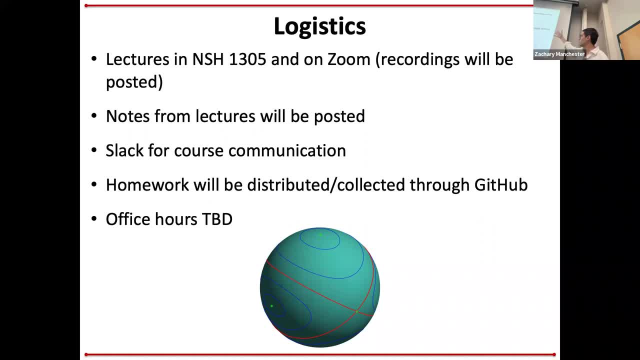 You can bug each other. Homework will be done through GitHub. It's mostly going to be like Jupyter Notebook stuff, And then we'll set up office hours, sort of TBD based on doing some polling of you guys. Any questions about this stuff? 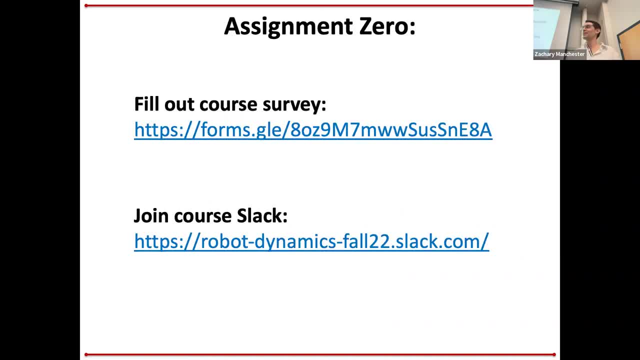 Straightforward, cool. OK, now you get to do something. So I think if we could all do this real quick, or at the very least snap a picture of this, or I'll post it. Number one is there's this Google form thing. 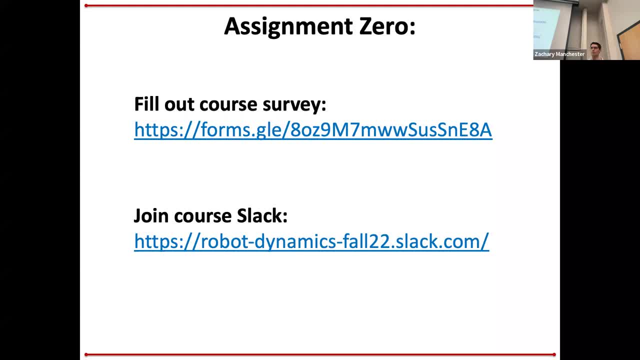 which is me bugging you about some questions about your background and stuff you already know about, and then stuff you're not You're into and want to learn about maybe. And then the second thing is just join the Slack, because that's where all announcements and things. 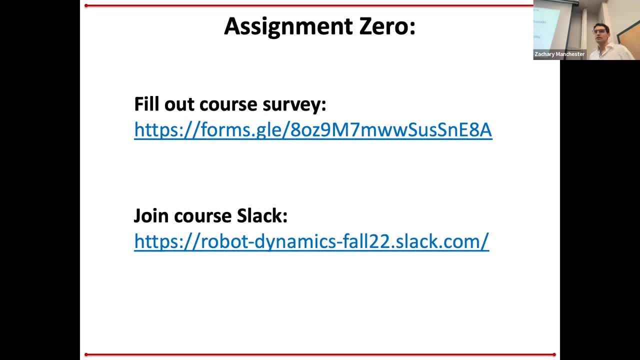 will be. I'll leave this up for a second. Hopefully you guys can grab those links. OK, we're pretty good. Yeah, All right, Cool, That is it for the introduction. Now I get to try to make my iPad work. 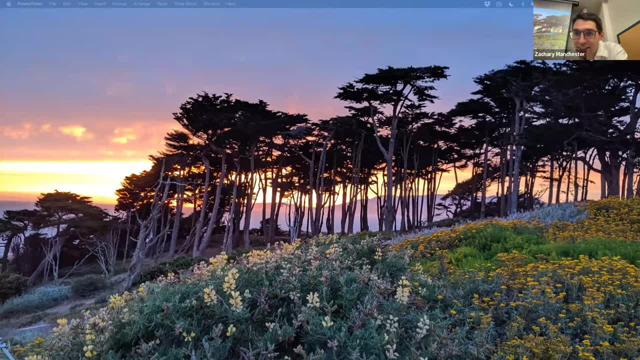 I don't know if you guys can see me. I'm not sure it's working. I don't know It's working. I don't know It doesn't work. It's not working. You can see me, It's not working. 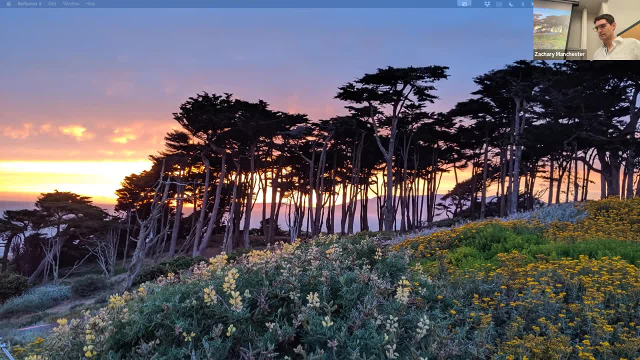 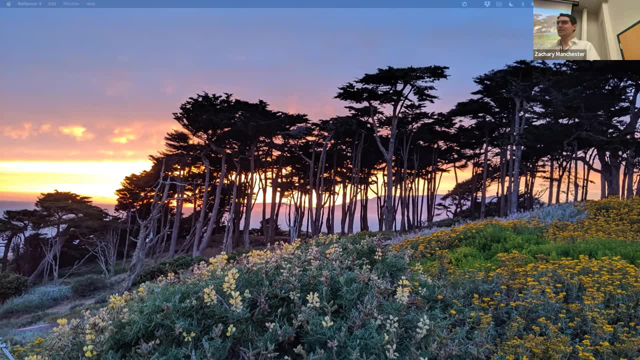 sorry. Okay, I did this last night at home and it worked. let's try again. okay, That picture is beautiful. No, Yeah, there you go. Do you know what the lines on it are called? Okay, yeah, yeah, you got it. 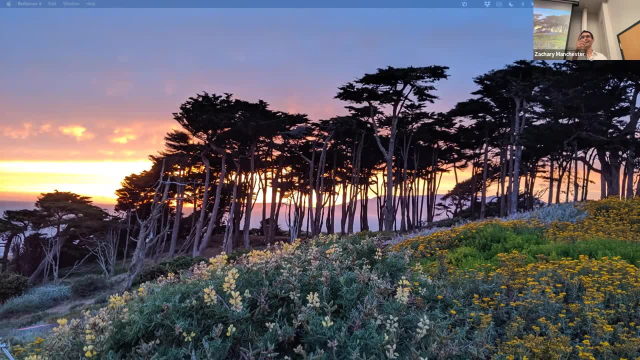 That's the. so yeah, that's yeah, you win, you win a bonus, bonus prize- as yet to be determined- bonus prize. So yeah, that is the. so if you take a rigid body that you know tumbles or whatever, 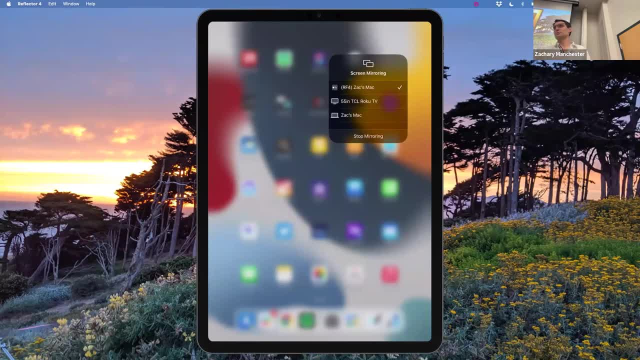 in general right, and you don't exert any torques or anything, angular momentum is conserved. So angular momentum is, you know, the norm of the angular momentum vector is conserved. so a constant norm vector in R3, it's a sphere, right? so what that tells you is going back. 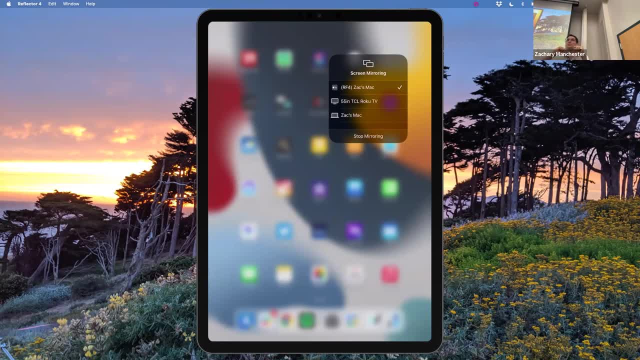 to this geometric mechanics stuff is that the trajectories for that rigid body have to lie on the surface of that momentum sphere, right, because of conservation of angular momentum. So those lines are a bunch of trajectories of a tumbling rigid body. They look like you know random tumbling, but when you look at it on that sphere it 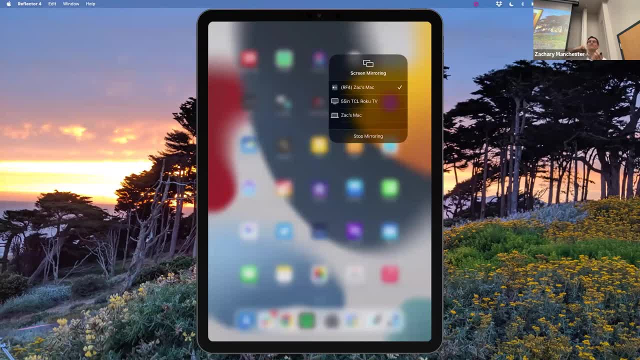 actually cleans up super nicely and they look like little Pringles slices- The red lines which now you can't see it. so this is like we'll do this. the red lines are fancy things called separatrices that we'll maybe talk about later. it's kind of 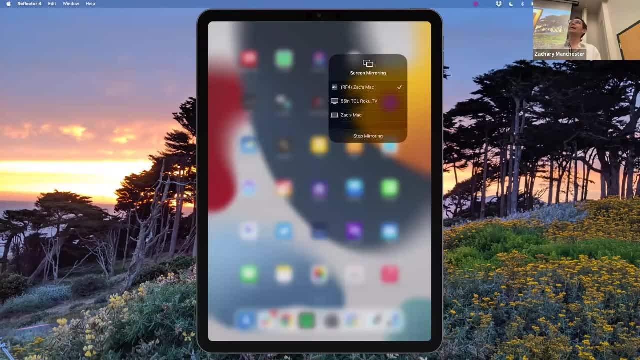 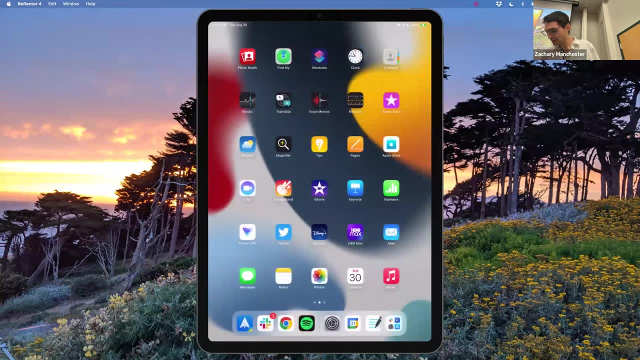 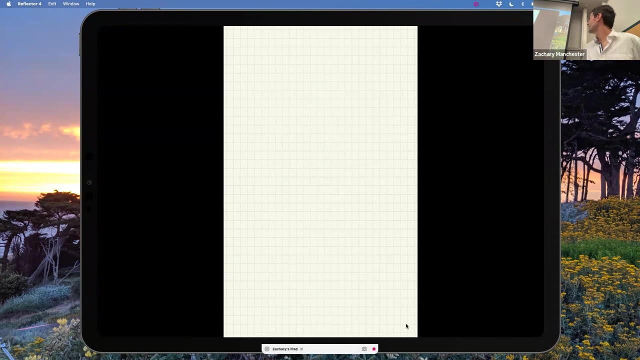 fun. They're also called homoclinic and heteroclinic connections, Okay. So you know, if you want to be super fancy, that's like that, geometric mechanics sort of lingo- Okay, I think it's going to work, guys, I think I believe. okay, anyone see everyone. 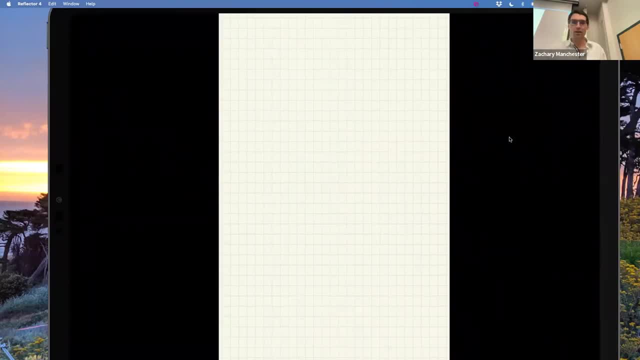 see this. okay, Yeah, we'll give it a shot. okay. so here's let's. so I figured we're going to start off. and yeah, why, why is this so awful? Okay, We're going to start off like nice and easy, keep things light today and sort of do like 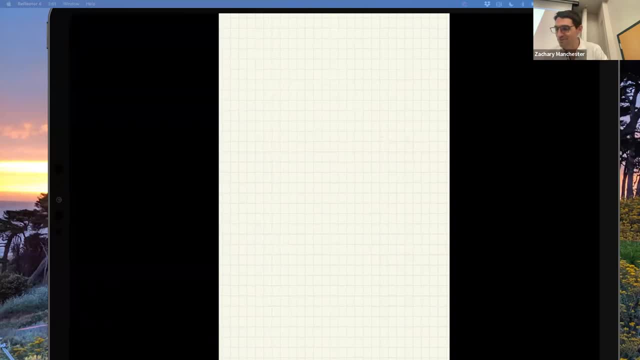 a little Newtonian mechanics review. so this is, like you know, F equals MA- stuff that I very much expect everyone to know, and I'm just going to kind of highlight a few topics of interest and like point some things out and then where we're going to go next time. 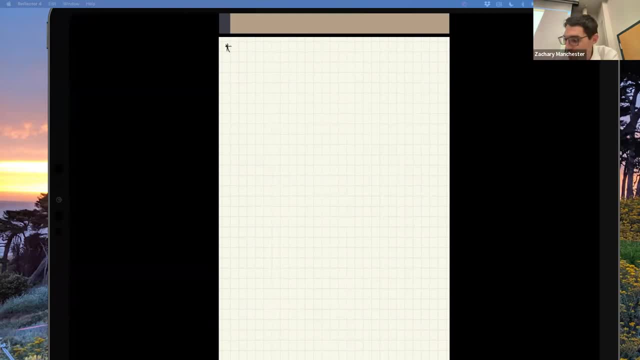 I think should be generally new for people. So, And again, I'm going to post this stuff online too, so don't stress out about copying down all my horrible scribbles and stuff. I'd much rather you, like, bug me with questions and 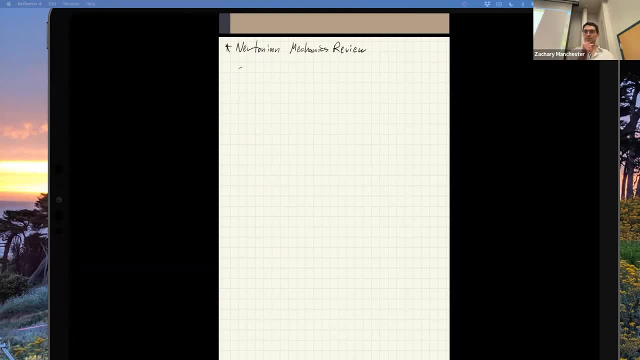 speak up and stuff. Okay, so the the Newtonian mechanics thing, the classic F equals MA thing. what that really is is about is describing the motion of particles, Or aka point masses. So, and what we mean by this right is things that have mass but no physical extent, right? 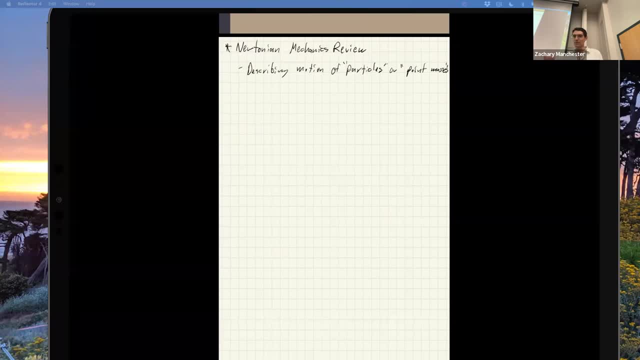 no volume, just like infinitesimal little points of mass. that's what F equals. MA is about. So when we say particle, There's a, There's a particular like mathematical meaning to that which is when we talk about, when we talk about writing down like the configuration or state of a particle, the 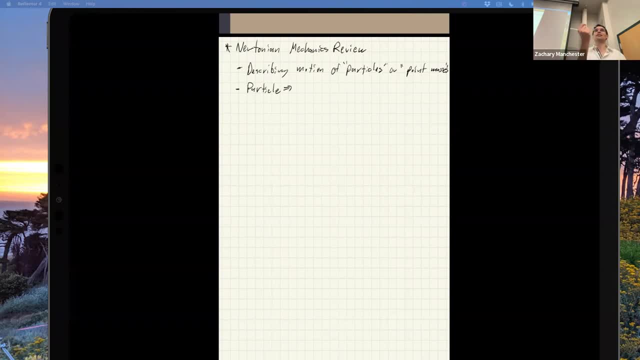 only sort of information we need. there is a position, a single position, vector right to describe the you know kind of where this thing is, its configuration right. And for now we're going to write that as a little vector guy like this. 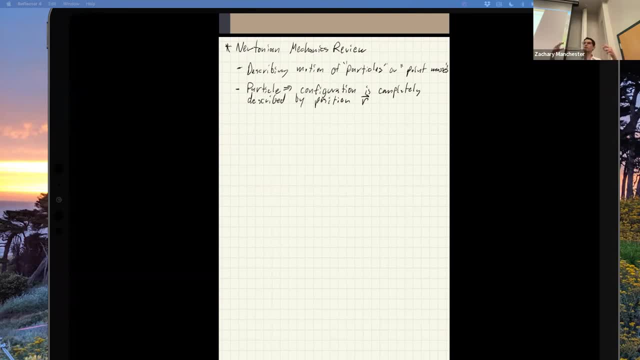 And if this thing did have some physical extent, right, if it did have some volume or whatever and took up some space, just a position wouldn't be enough anymore, right, We'd need some more numbers in the configuration to like uniquely specify you know where. 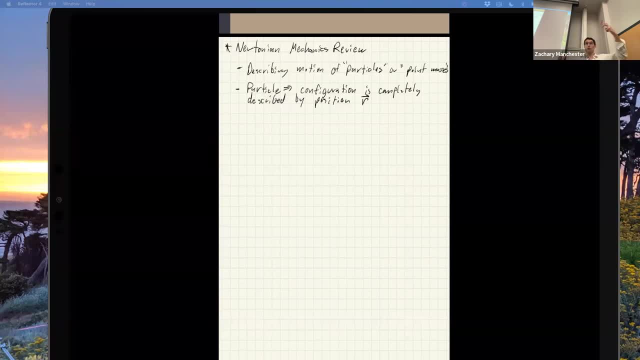 this thing was and stuff, right. So, in particular, right if it had physical volume and it was a rigid body. now it has a position and an orientation, right. So now we need, you know, more numbers. If it's a non-rigid body, it gets even more complicated and you have to write down like: 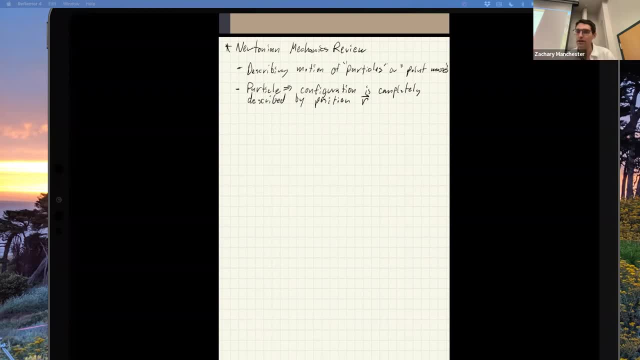 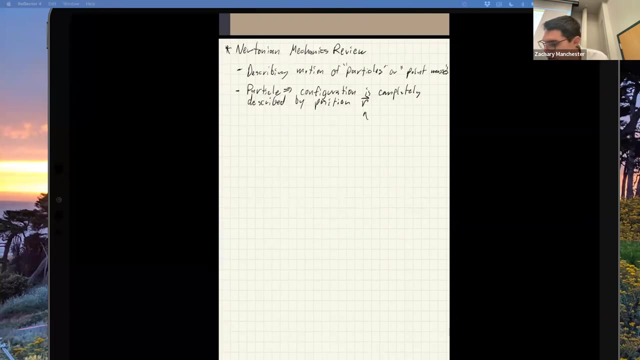 you know the configuration of various bending modes and stuff like that, right? So point mass means or particle means, it only has a position, Right. And then to sort of like just some notational things, This guy here, because it's going to sort of, we're going to play some games with coordinates. 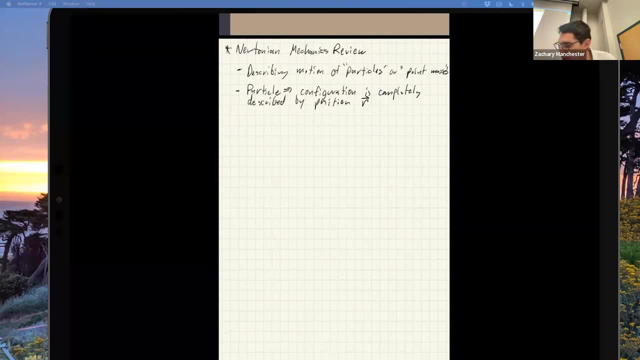 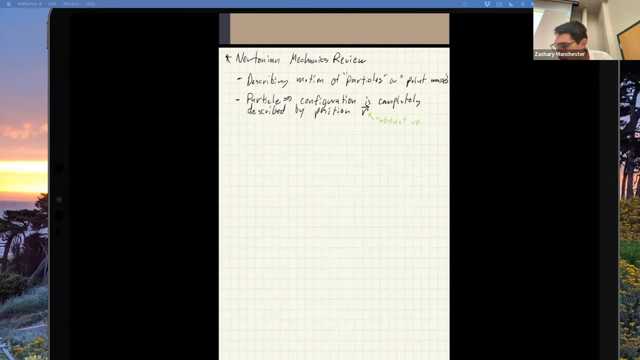 This r with the little vector guy on top. we're going to call this an abstract vector, And so we are. The meaning of that will be hopefully clear in a sec. So abstract vector means it's not. it's not a set of numbers, you know, stacked up. 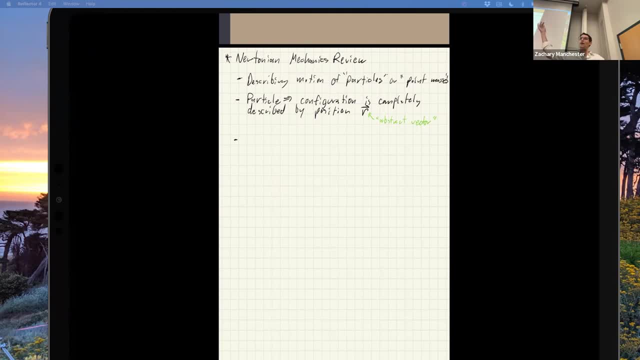 It's some, it's a, it's a like arrow out there in space without a coordinate frame attached to it, right? It is a like position thing, right? that's sort of an abstraction. It doesn't have sort of particular numbers attached to it. 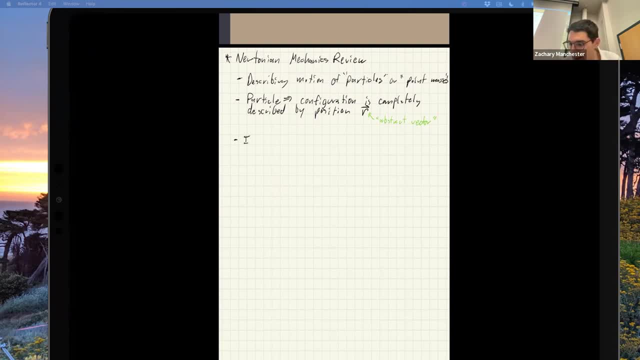 That's what I mean by that. So we can write down: F equals ma in this sort of coordinate-free form, ie in terms of like these abstract vector things that don't have numbers, that are just kind of little arrows. 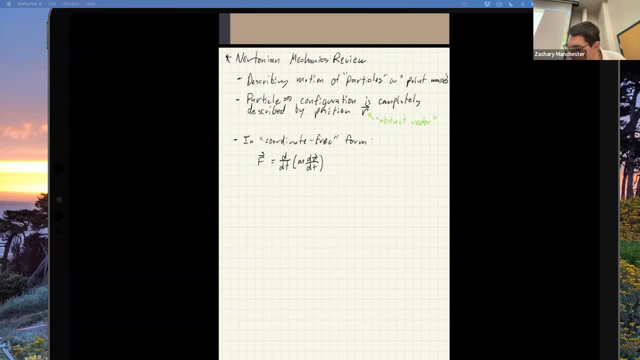 So this is Mass right And if we assume- And then the other thing is velocity in there We're going to be sort of like super pedantic for some of this stuff to like get mutation down. This guy in here is the velocity now. 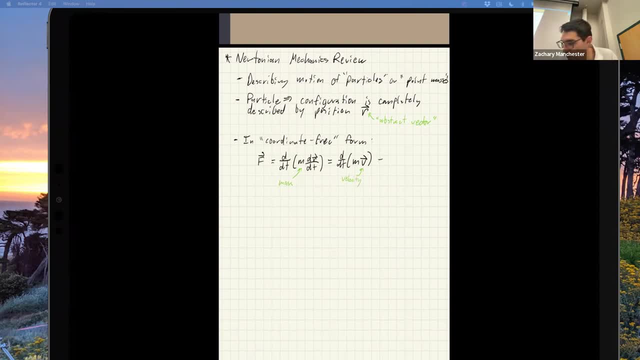 Also a weirdo abstract vector, This whole thing, And v in there is the time derivative of the momentum, and this is all stuff that I'm sure you guys know. Okay, so if we assume that the mass is constant, which isn't always the case, and there's, there's one problem where it's not, that's like a classic, which is the rocket equation, which is a fun one. 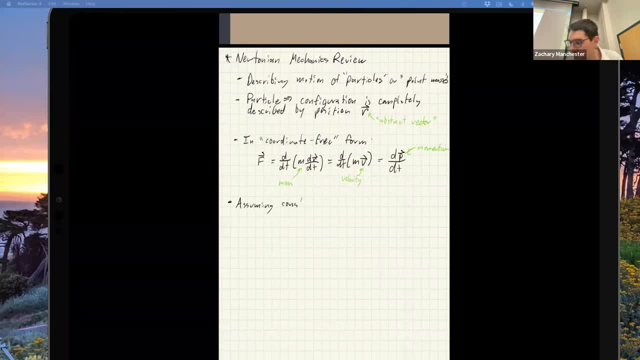 Okay, so if we assume that the mass is constant, which isn't always the case and there's, there's one problem where it's not, that's like a classic, which is the rocket equation. which is the rocket equation, which is a fun one. 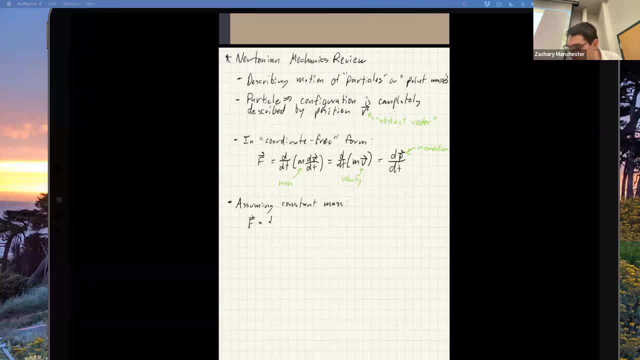 That we get. You can pull the m out And we get the classic F equals ma thing, right? Okay, so this was all in sort of weirdo abstract vector land and we can't actually do anything with this at this point, right? 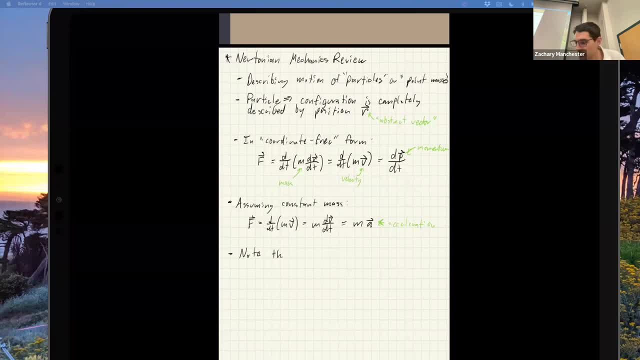 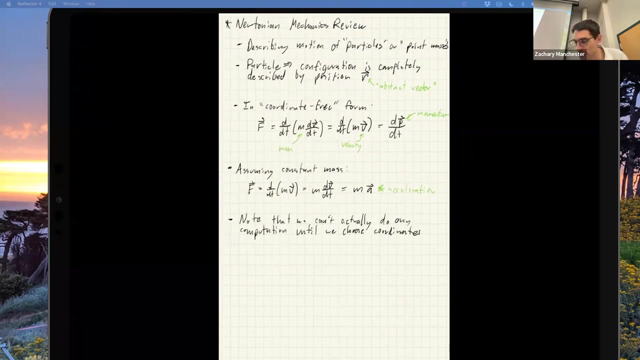 So write that down. We can't actually do any computation Until we choose coordinates, So we're going to be like super explicit about this, at least for a little while. So let's pick some coordinates, and the the most classic choice would be Cartesian coordinates. 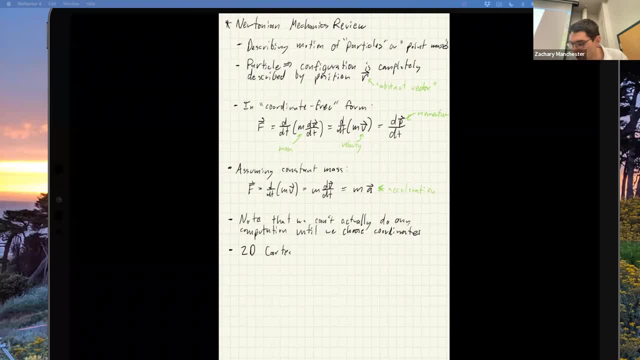 So let's do just like in 2D for now. So we're going to- We're going to take this position, vector r, which is this abstract arrow thing, and we're going to resolve it into standard xy Cartesian coordinates And the way that looks. we've got a, say, an x component, which is a scalar, and then we're going to have these unit vector things. 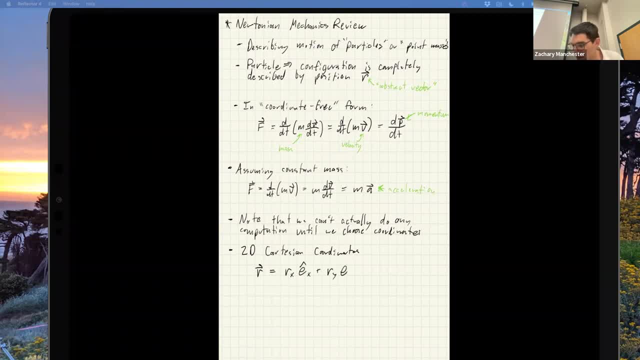 So this is the x unit vector, and then we're going to do the same thing with the y's And I expect like you guys have seen stuff like this before. So we've got These things which are scalar And we call these components right. 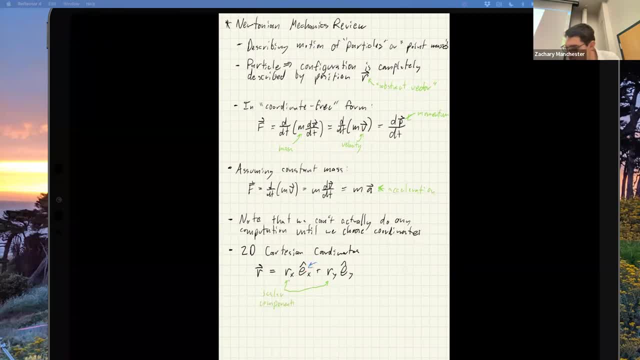 And then we've got these things which are vectors, unit vectors, And these we call basis vectors And another way of writing this down. right, You can think of this expression as sort of like a dot product between Some sort of you know the standard thing, right where I stack the components into a thing we're used to calling a vector but is really, you know, not a vector in this more sort of abstract math sense. 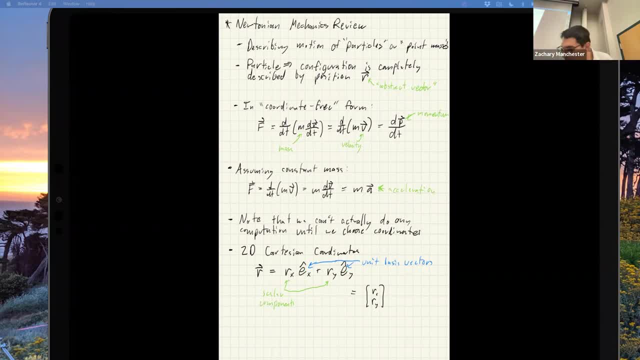 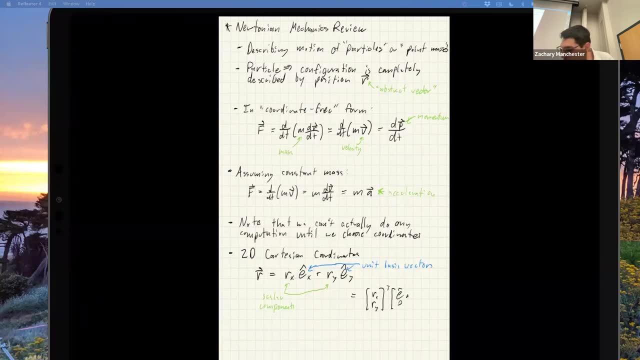 That's really a matrix of components. So you can think of it like this kind of idea: You have like the components And then you have the basis vectors And the abstract vector over here is like the dot product. It's between the components and the basis vectors. 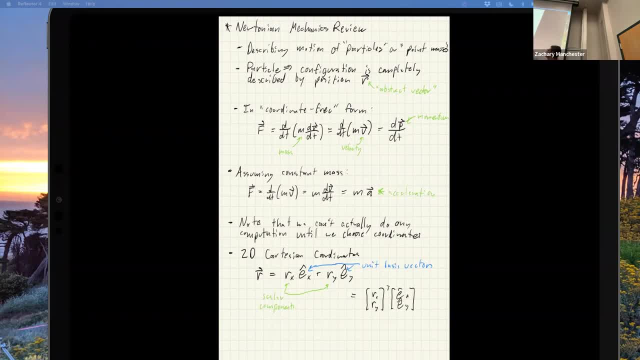 Right. Does that make sense to everybody? This is sort of actually kind of a I don't know An interesting notation. These are sometimes It's called a vectrix sometimes, which is kind of a weird thing. This is kind of standard in the aerospace community where you have to like reason about lots of coordinate transformations all the time. 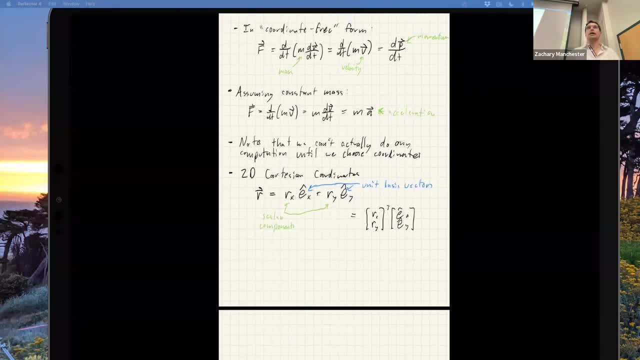 Okay. So what happens now? if I take this thing, I want to diff this to get v, let's say, like we had up there, So I can say: you know, v equals dr dt And I can just go ahead and diff that expression. right, that coordinate frame expression. 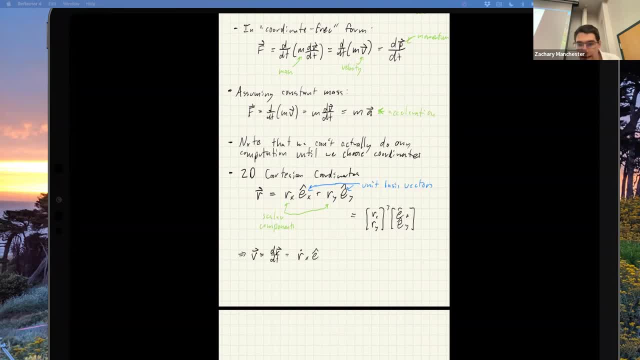 And I'll get like r dot e, hat x plus r. Okay, Then, like the time derivative of the basis vectors, Right, Right, And a sort of obvious thing happens here, which is that the time derivatives of these basis vectors are 0.. 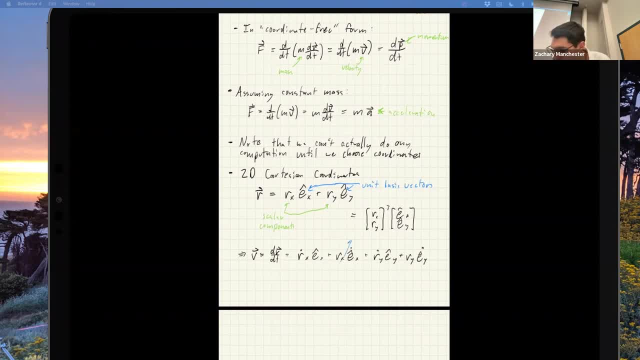 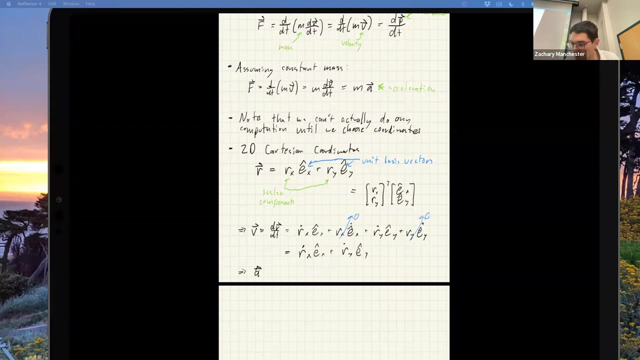 They're just sitting there, fixed, So we can drop these guys out, Okay, And this then reduces to sort of the obvious answer, which is just: you know the stuff you're used to seeing, And you can kind of do this: you know again and get the accelerations. 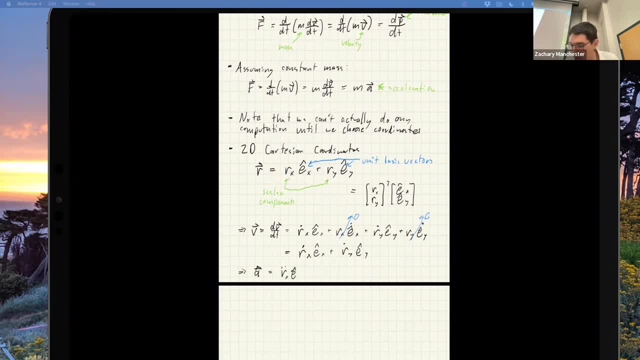 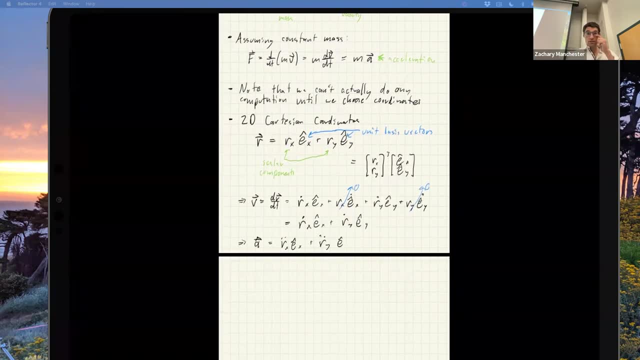 And that's sort of again super straightforward because things- The basis vectors- are constant, So no surprises here You get this thing, And so it turns out that if we want to write f equals ma down in Cartesian coordinates, we get the standard thing you're used to. 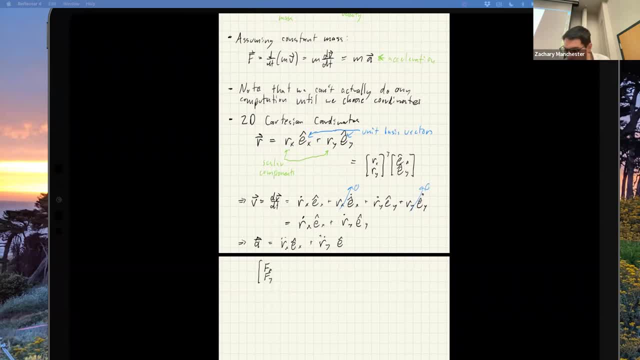 So if we want to be super pedantic about the coordinate frame stuff, we'll get again the abstract vector stuff. So I'm going to do the f in Cartesian components And then the ma, Again Cartesian stuff, And I'm going to keep the basis stuff around right. 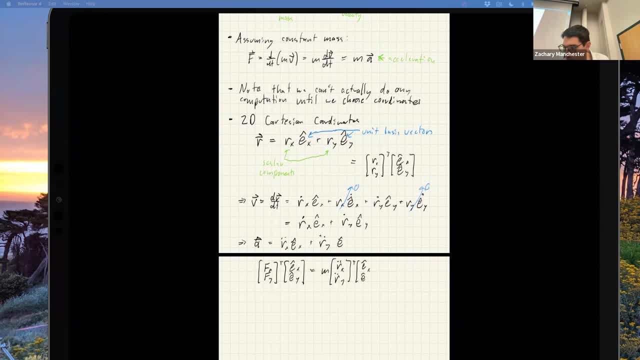 This is exactly the abstract vector equation that we had before. Kind of the idea is, I can stare at this and I can say, okay, well, I can just pull these off. These are the same on both sides, right? So I'll just keep the component equations. 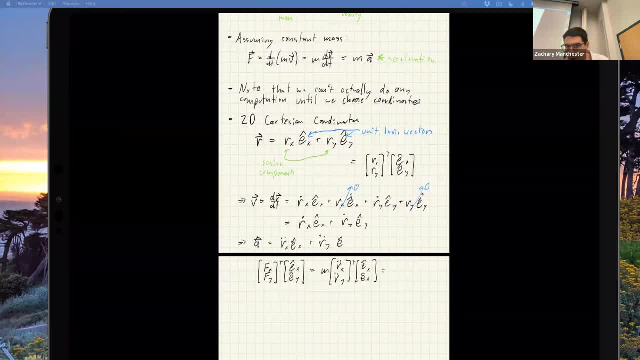 And that's you know kind of how we get the equations. we're used to seeing Where we're dropping the basis vectors and just looking at the components. So I'm being like extremely So I'm belaboring this component stuff versus basis stuff- a ton. 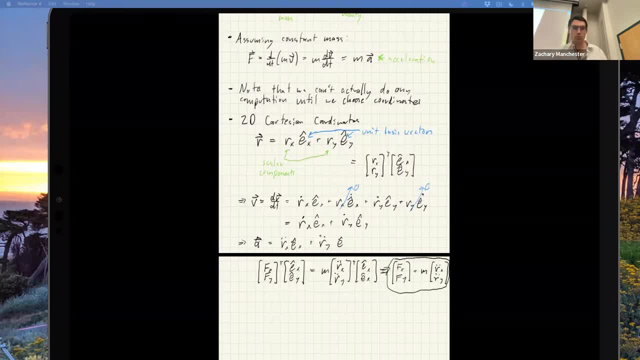 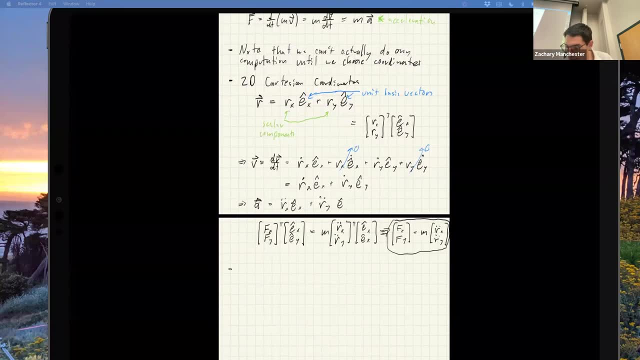 So this is kind of the thing we're used to dealing with, because what we're going to do next is not Cartesian coordinates. So if I make a different choice of coordinates- which is a normal thing to do, Let's say I You go for polar coordinates instead. 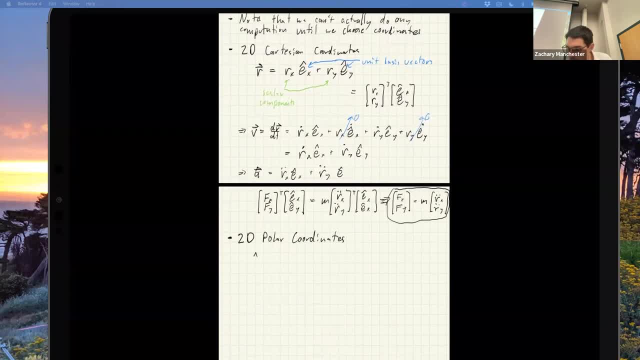 Let's write those down. So I'm going to start with my Cartesian coordinates. So I've got my x basis vector, y basis vector. Then I'm going to write, like I'm going to write down some, you know, just kind of arbitrary vector r: 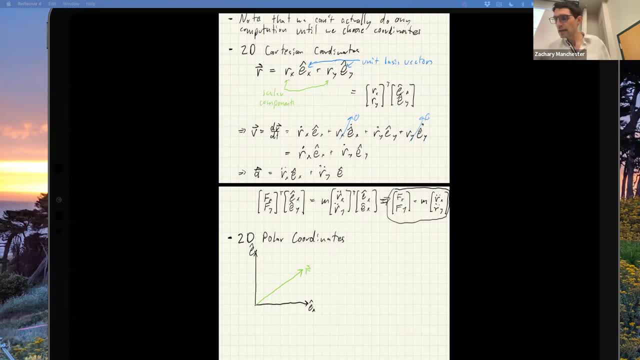 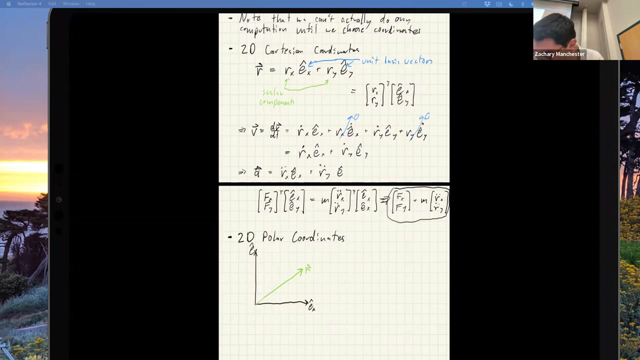 Abstract vector-y thing, whatever. And now I'm going to write down the polar basis vectors. So I've got the components in polar coordinates right as r and the radius and then theta, the angle. So if I write down the basis vectors for that, the r one is super obvious. 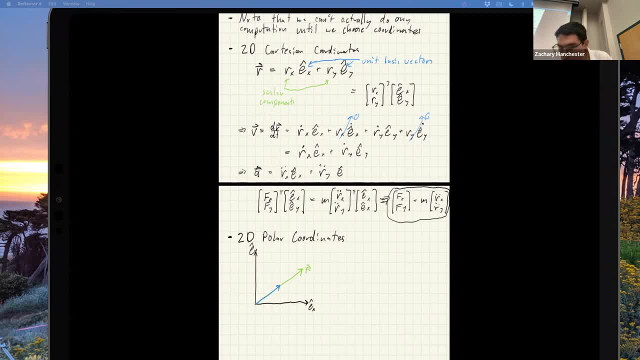 The r one is just the unit vector along here, right? So this we're going to call e hat r. And then what's the theta basis vector? Yeah, exactly So it's still an orthogonal basis. blah, blah, blah. 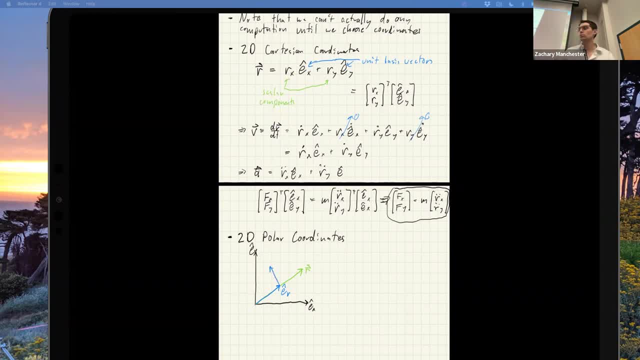 So it's, yeah, the unit vector perpendicular to that one. So we'll call this: e hat theta, Let's write these guys down. So what we're going to do now is write down, like the conversion between polar and Cartesian. 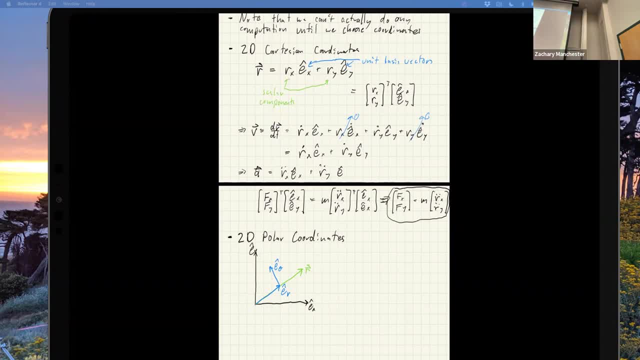 So what we're specifically going to do is write down these two basis vectors in terms of the Cartesian ones, So we have the mapping back and forth. So if I do that, this is like I'm not going to spend a ton of time on this, because this should be. 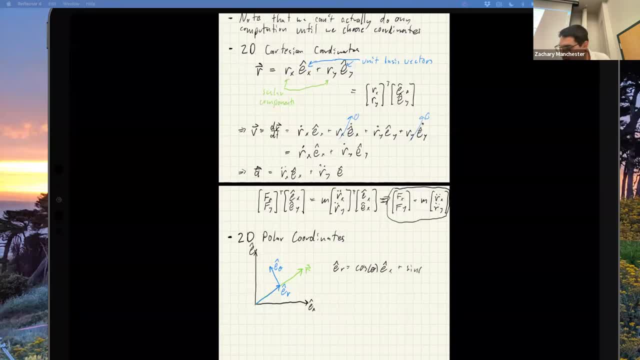 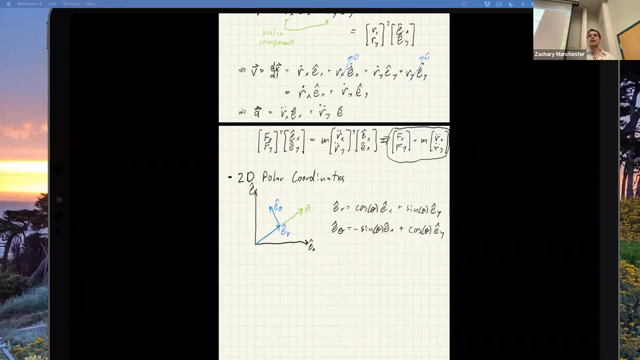 You know you can stare at that and do a little trig. It's not too hard, Okay. So that's that. So here's where it gets weird. Now I'm going to write down like I'm going to try to take that r guy's derivative. 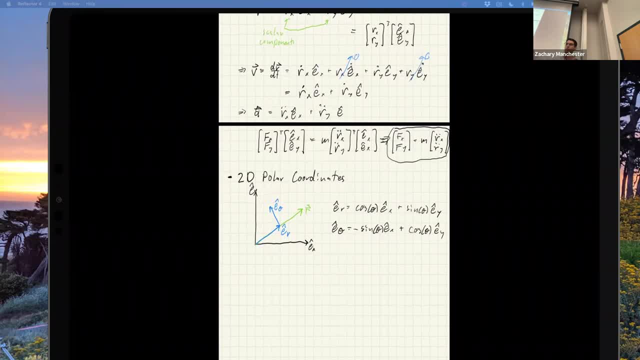 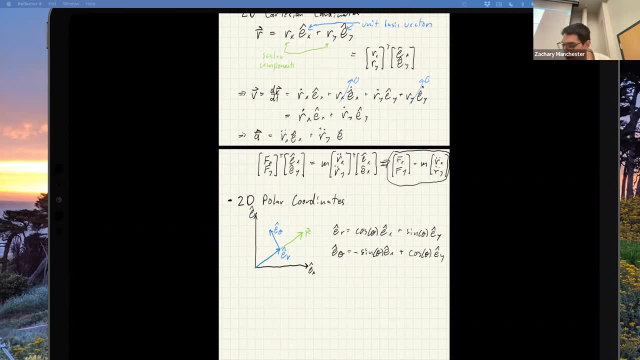 I'm going to try to write down r dot in polar coordinates. now, right, And what happened before? you know, everything was nice, The basis, vectors were constant, vectors were constant and dropped out, and then you got this really clean expression. Let's see what happens in polar coordinates. So if I write this guy down in polar coordinates, 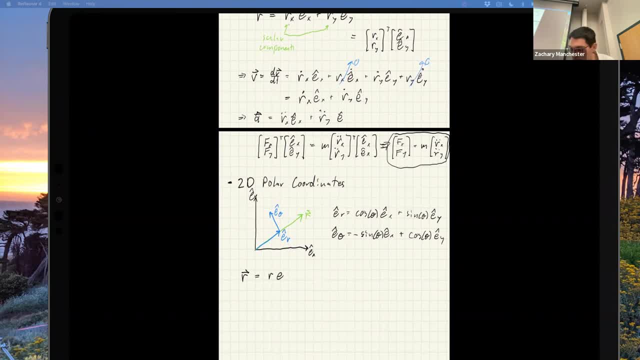 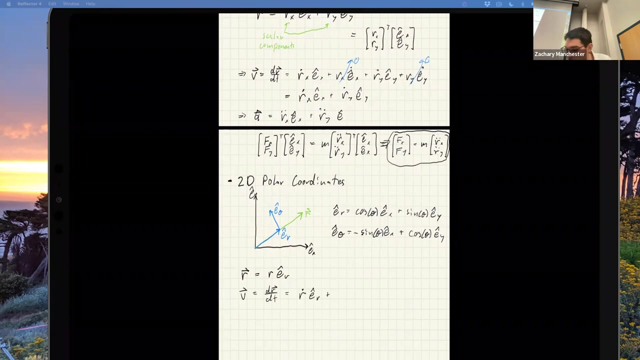 this is just scalar r times e hat r always right by definition. basically, Let's try to write down the v vector now. So this is dr tt and I'm going to expand this out. I'm going to just do, you know product rule. So I'm going to get r dot e hat r plus r dot right. 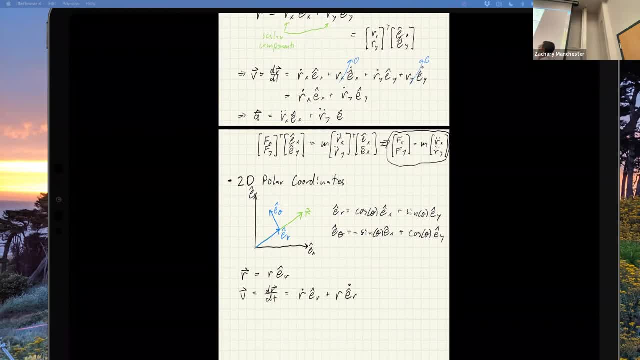 Last time that was zero. but just by looking at this right, if I move r around, this basis has to move too. So what this is kind of showing you right is, as r moves, these basis vectors are also changing in time, So that this guy, this basis vector derivative. 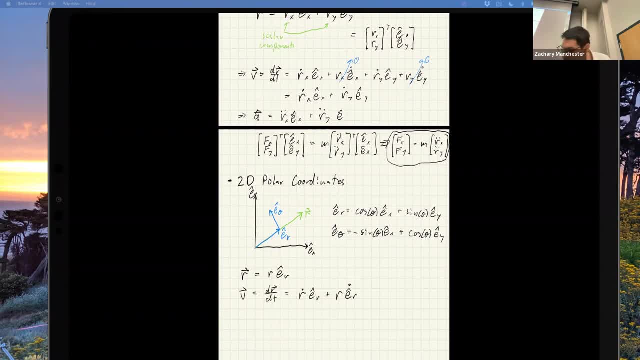 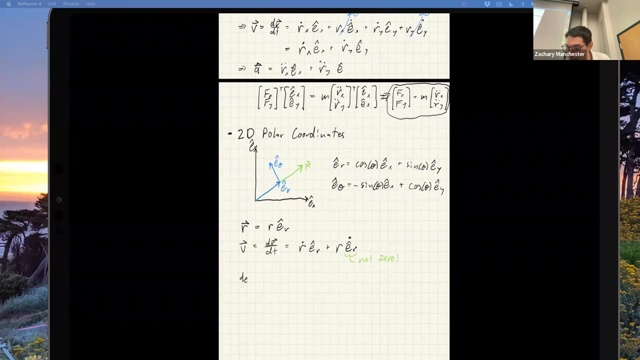 is going to move in time, So that this guy, this basis vector derivative, is going to move in time, no longer zero. We have to like kind of pay attention to this And it gets messy. So I will like I guess we'll go kind of fast and not be sort of 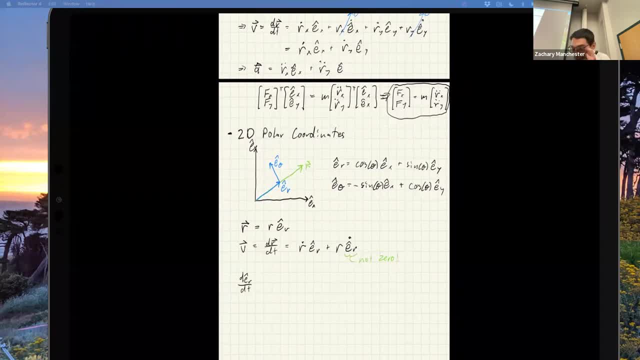 I mean this is easy, you know freshman calculus stuff. It's not not too hard, but we'll write it out. So I'm going to just plug in the definition there of like this guy in terms of the Cartesian coordinates, because I know. 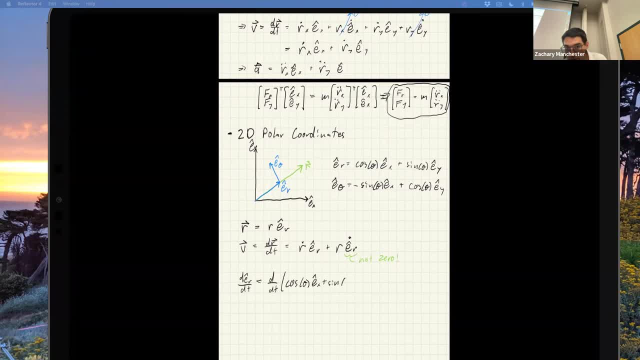 those are constant and I know how to deal with those. And now I'm just going to diff that Getting terrible. I should move this over, Okay, and if I like, sort of like stare at that minus sign post, that looks like this guy right. 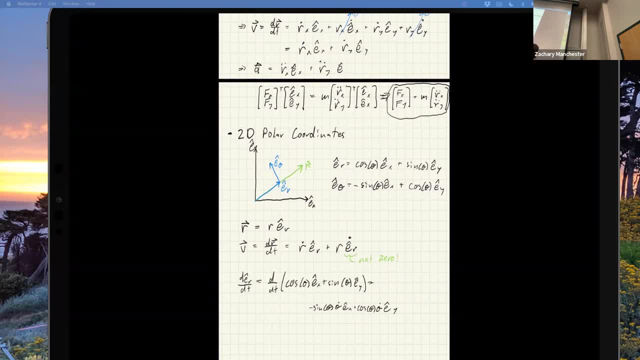 So that's this minus sign. you have x post, you have y, that's the. you have theta basis vector, right? So this guy is actually theta dot e hat theta, which kind of makes sense, right? So if you think about this, 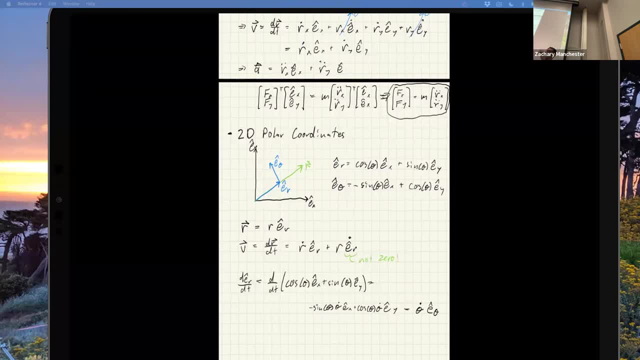 if this thing's moving at all. at this e hat r guy it's moving like that, The only. so if it moves in the radial direction, the e hat r doesn't change at all, right, Because it's a unit vector. So the only thing that can change is if it rotates a little bit. 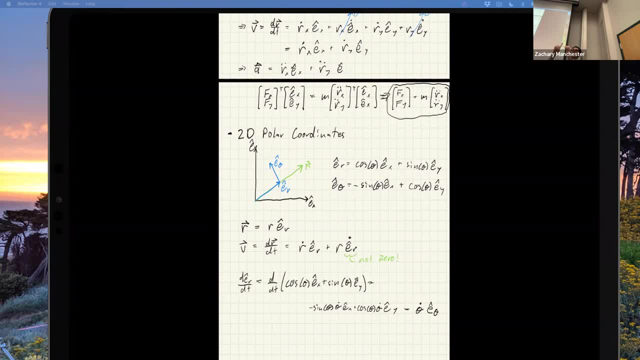 right. If you're moving any other way other than radially, any change in that guy is going to be is got to be perpendicular to the e hat r. Does that make sense? So, like intuitively from geometry, like that's, that's got to be the answer. 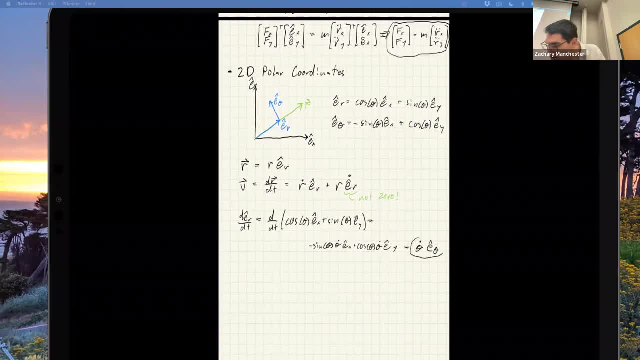 Okay, so we figured that out And now, now, right, we're. so. the game here is: we're going to try to write down: f equals ma. That's where we're going in polar coordinates. So we got to do this one more time. 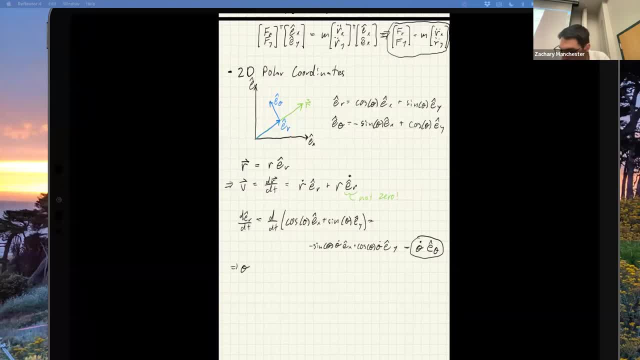 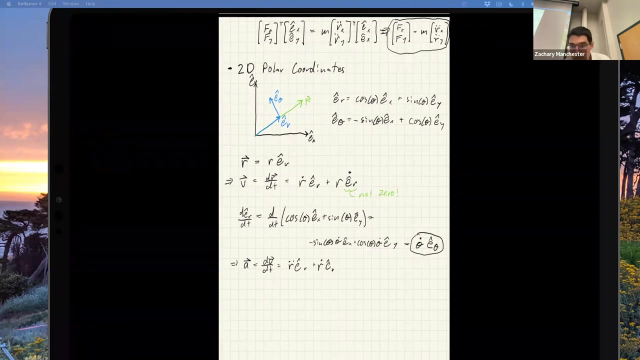 So now we're going to do the a, Okay, So. so I'm just going to do this guy again, Okay, Okay. and now we're going to start like simplifying things down. The first term stays No weird stuff there. We're going to like like start collecting some things. 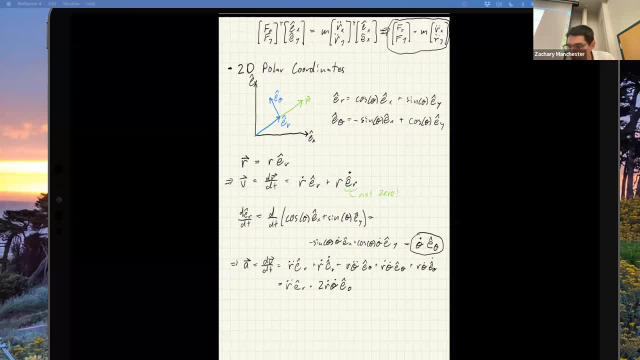 And like pulling out some stuff. So what? all I did was go and plug in, like this guy, that I already do right, and this guy go figure out the same way. So the upshot is, if I take this now and, like you know, plug into f equals ma. 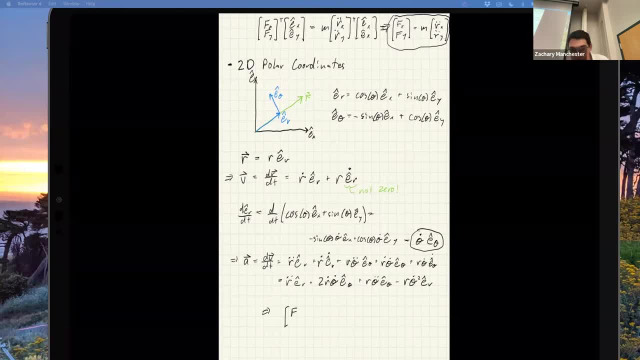 I get this like pretty gnarly-looking component. you know sort of definition for f equals ma. Okay, that's f equals ma in 2d polar coordinates. That's kind of awful. So the the main takeaway here is that 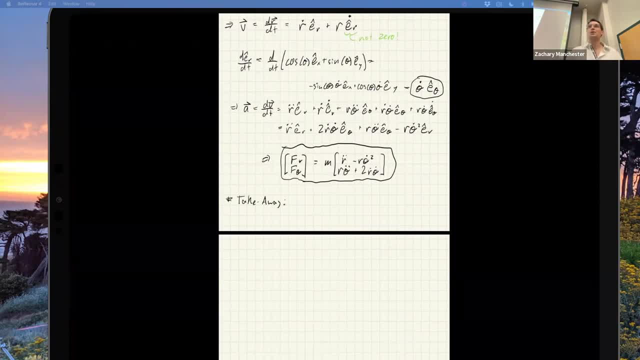 sort of. the reason for doing this is to, you know, give you a taste of the suffering that is trying to do. f equals ma on slightly complicated systems, And you know the Newtonian sort of formulation: the f equals ma thing. 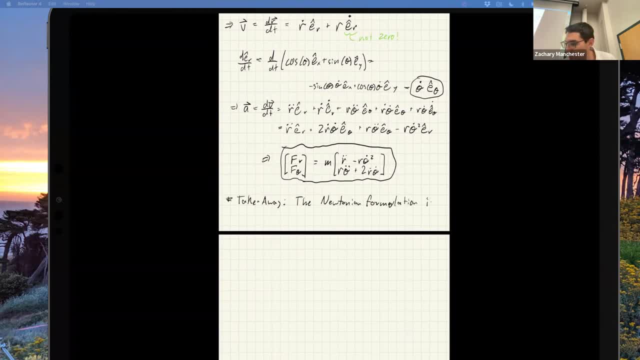 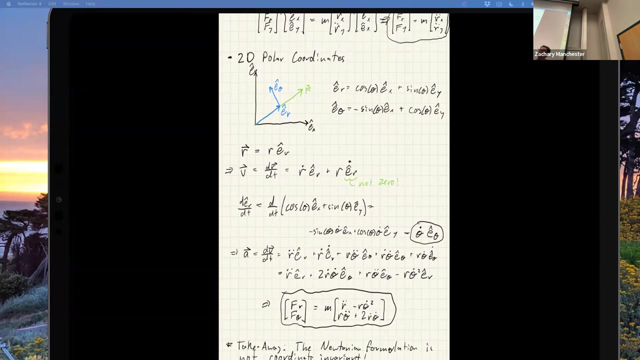 you know the Newtonian sort of formulation: the f equals ma thing is very much not coordinate invariant. And to make that clear, right, so what? what we specifically mean by that is that the equations of motion in a particular set of coordinates is completely different, right? 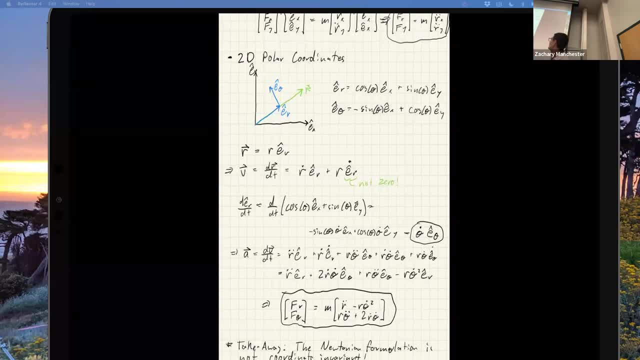 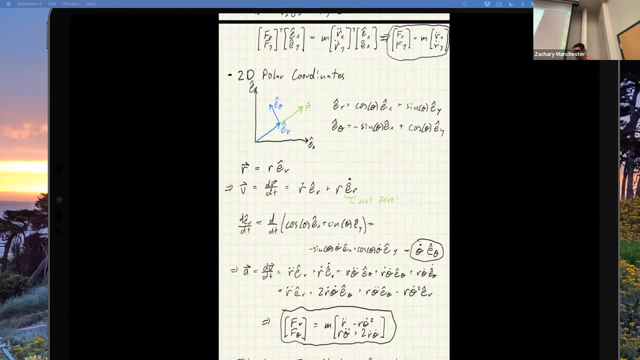 So here this does not look anything like the Cartesian version up here, right, Super different expression And coordinates, right, And that's in contrast to the Euler-Lagrange thing which you know, with the q's in it. 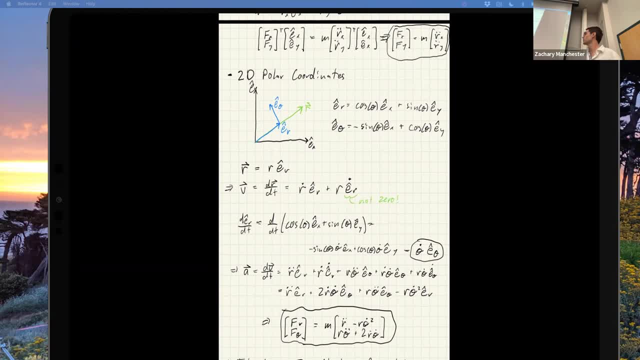 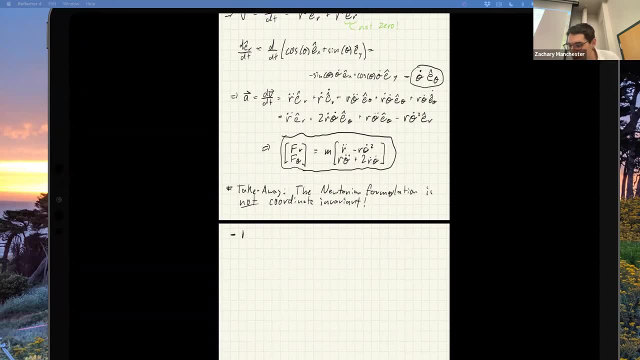 which is the same in any coordinates you want, right? So that's kind of the big deal And sort of like. the corollary to that statement is that this becomes really unwieldy for anything you know more complicated than like. 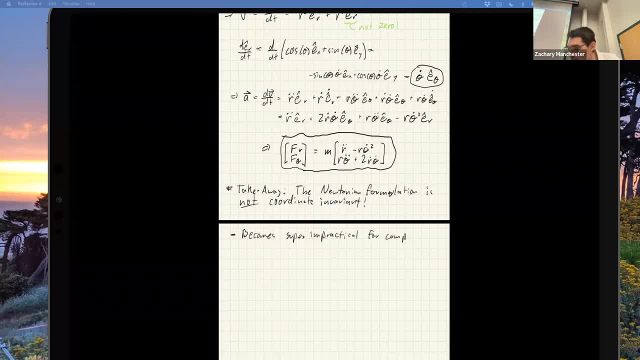 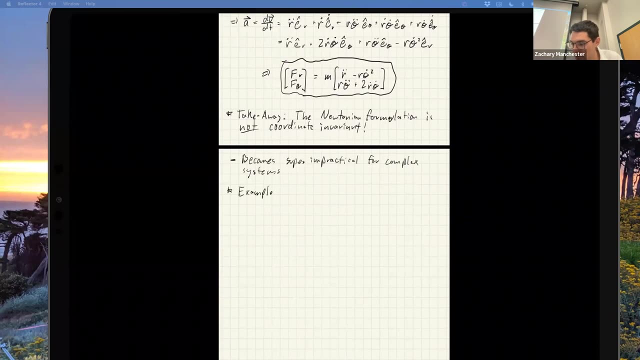 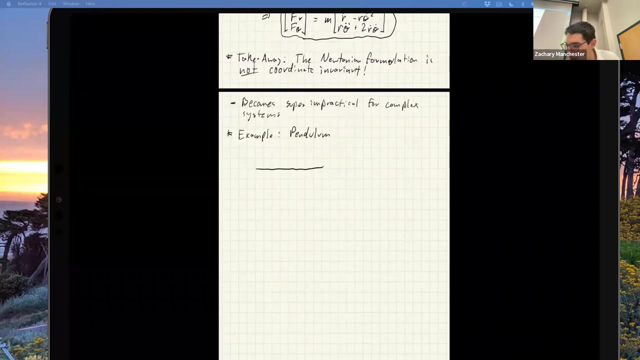 a pendulum or whatever. So let's do the pendulum, Why not? Okay, so everyone's seen this before, So what we're going to do is so we can like write down. you know our like. 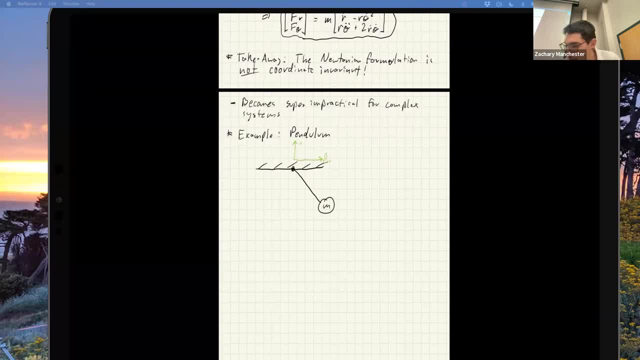 Cartesian basis here, And we can also write down, you know, our polar coordinates. So here's say, this is our theta, This is our l, And if we're going to do the like, f equals ma thing- we also have to think about, you know, the. 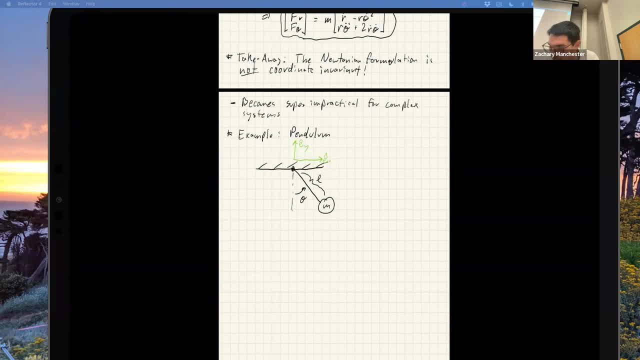 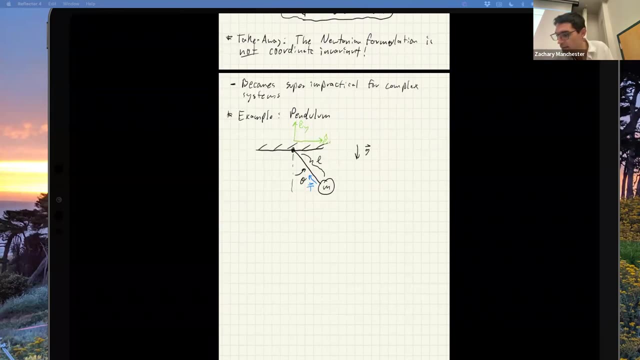 full 2d dynamics here. So we're going to also think about this tension force that acts in the radial direction, So as sort of a like I don't know hint of things to come. Oh, we got gravity down. 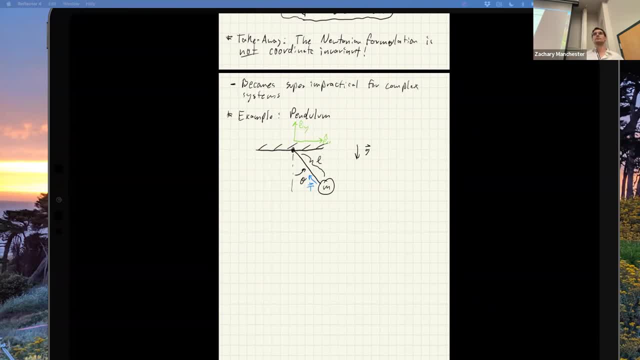 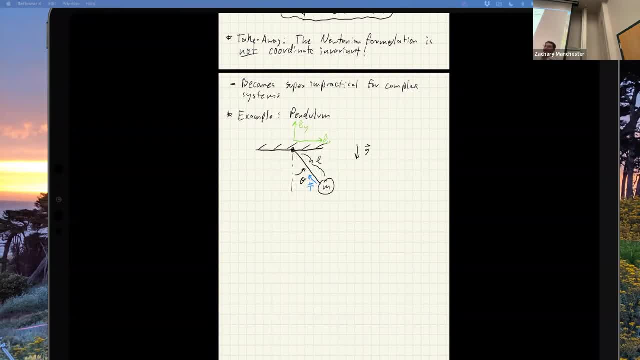 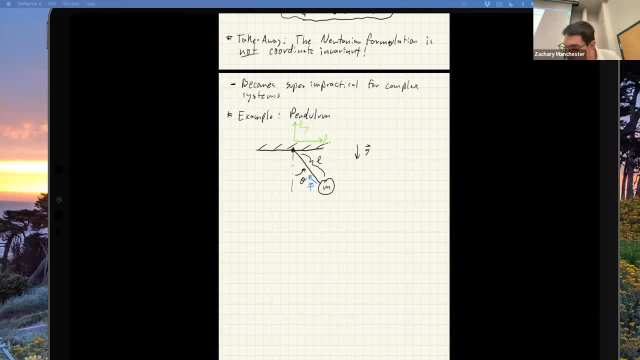 x and y, or r and theta, right. So if I wrote this in Cartesian coordinates, say, right, I'd have to write down two numbers to specify that guy's position, right, I'd have to write down x and y. So one way of thinking about this is that you know it has 2d of f. 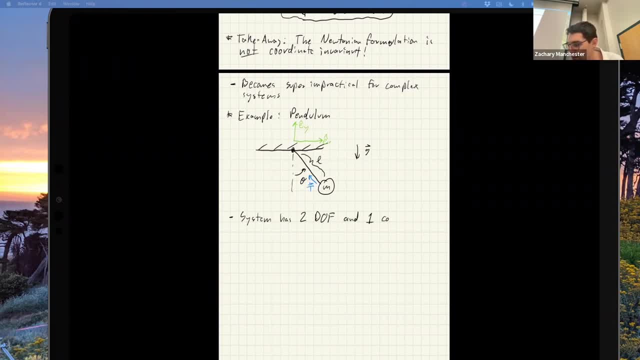 and one constraint. So it has basically the following: So this position, vector r in 2d right, x, y, whatever The norm of that guy for all time has to equal l, that length right. Does that make sense? 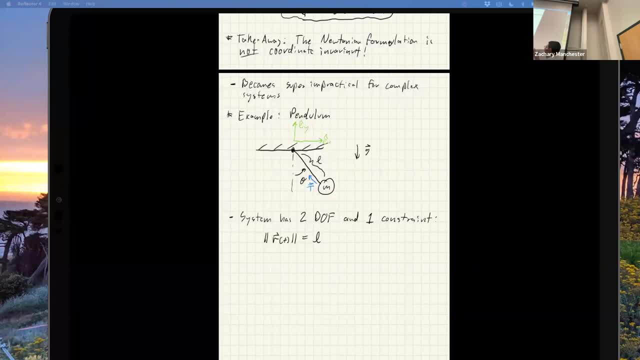 So that's my constraint. So in general I have some system I can write down, You know. so in this case, if it's a point particle in r2, the so-called maximal coordinates would be to write down, you know. 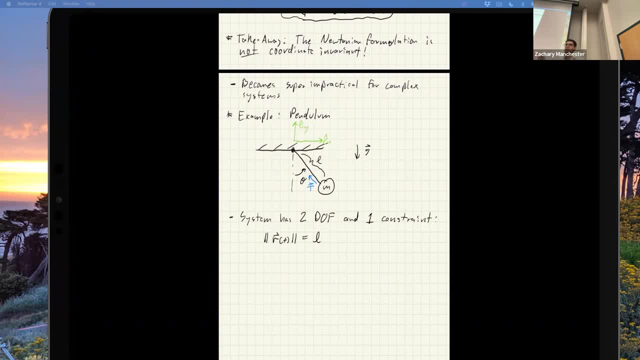 the full, like Cartesian specification of everything. So here that would be two position coordinates, x and y, And then you write down the constraints explicitly. So we'll do more of that kind of thing, But you have this constraint And then we could write down in sort of Cartesian coordinates, right? 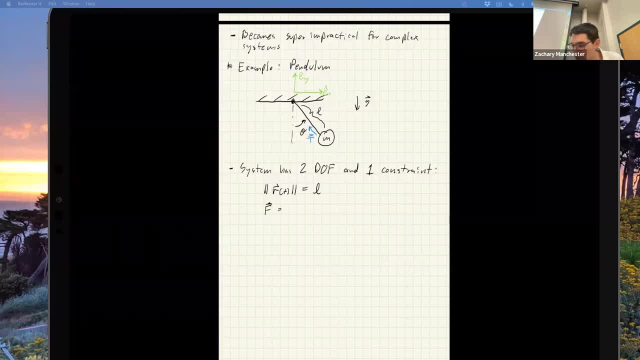 We can write down: f equals this tension force plus mg. Those are the only forces right. And this has got to be equal to m, v, dot or ma or whatever In Cartesian coordinates. I have to explicitly figure out this t. 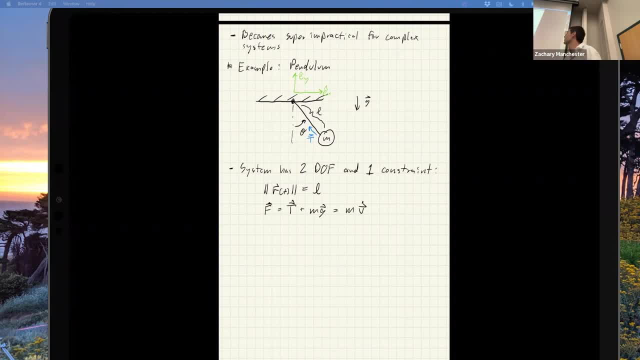 which is actually like coming from the constraint in some sense right, Whereas in polar coordinates it works out a lot nicer. So in polar coordinates. So in polar coordinates it works out a lot nicer. So in polar coordinates I can write down the radial stuff in components. 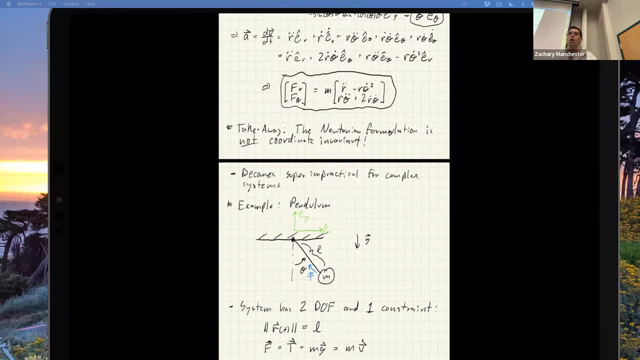 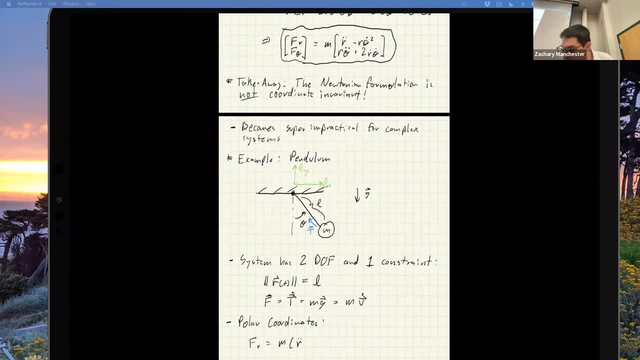 So if I go back over here, I'm going to just plug into the fr line from the polar coordinate stuff. So I get m r double dot minus r theta dot squared, What's r double dot Zero. right, Because I have that constraint. 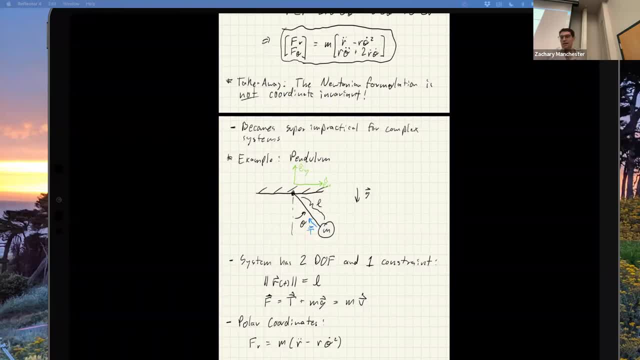 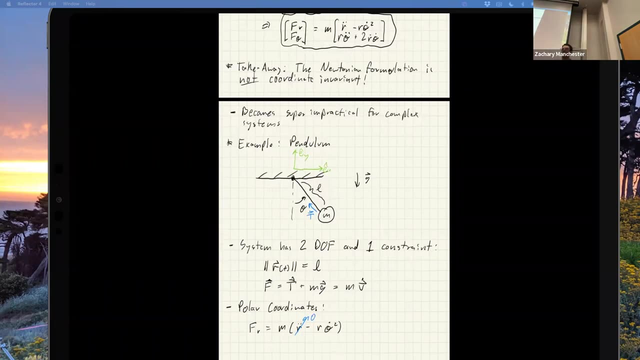 Because I have that constraint Right, So that if I diff that it's got to be zero. Okay, let's write down the theta equation, Also the r here. What's this r? L right? It's a constant. 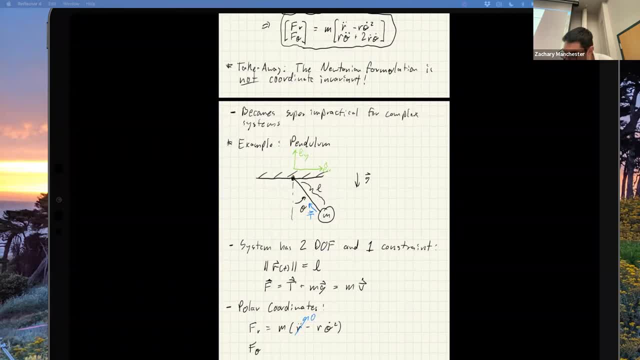 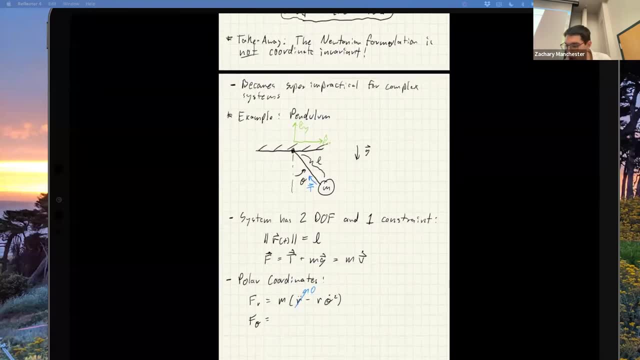 Okay. and then we got the other stuff, the theta part. Again, just plugging into that bottom line up there for f Theta There is. let's see what do we get? We get Okay, same story. We got an r dot here. 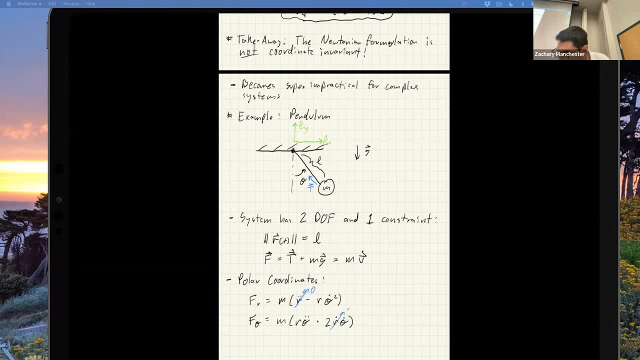 That's got to be zero, So that's going to drop out. So this simplifies down to m, and then, yeah, r equals l right, m, l theta, double dot. So from here I can say a couple of things. 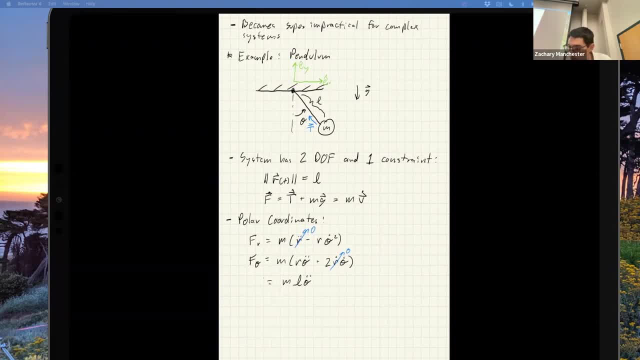 The first one is that t, the tension force is equal to minus t e hat r. So it's got to act in the radial direction. It's acting in the minus radial direction, right, Then I can write down gravity in these coordinates. 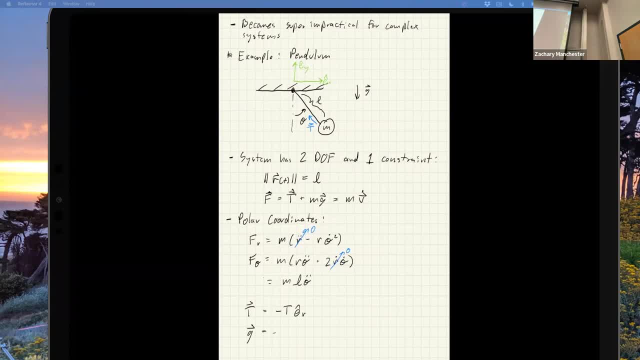 So what I'm trying to do here right is find that mark. So this guy is totally, this is going to be an f? r right. Then the gravity stuff. if I resolve that into you know a t, that into like cartesian coordinates, it's purely, it's minus g in the y direction in cartesian. 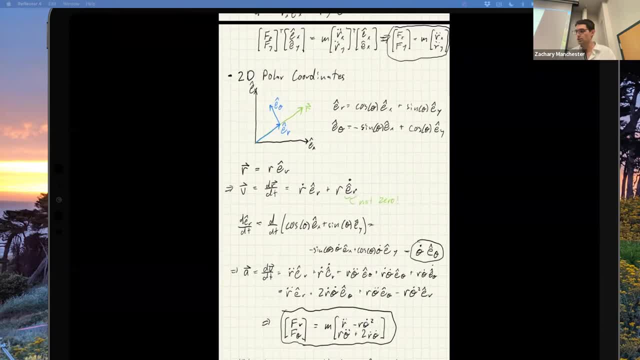 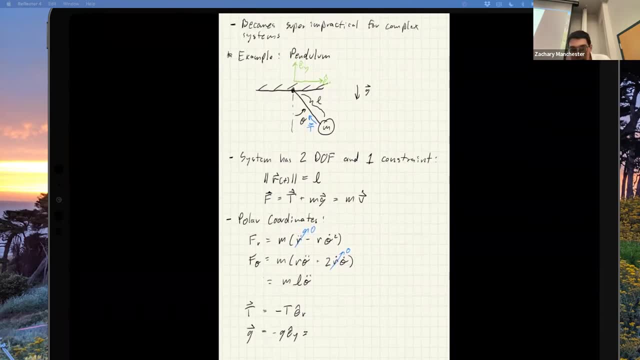 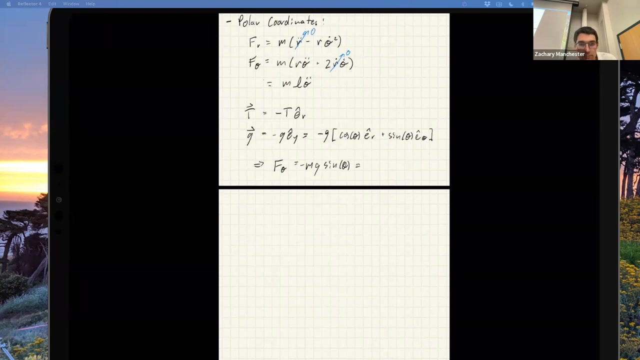 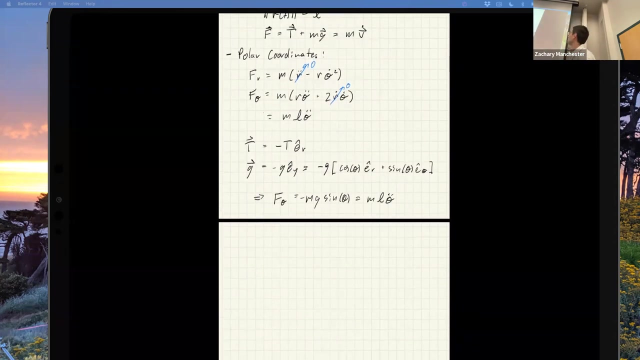 i'm then going to go plug in this coordinate transformation right between the r? theta and the xy stuff, so i get minus g. okay, now i can sort of pull out this f? theta guy minus hold on. oh yeah, here we go. okay, so that's me pulling out the f? theta from the sky. 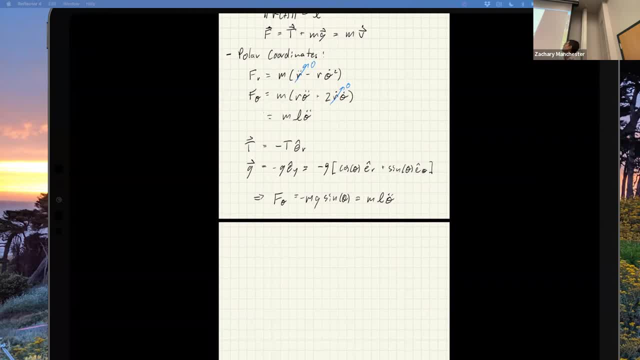 plugging into the theta equation. The r dynamics don't matter, because the constraints keeping r fixed r double dot 0.. The only stuff I care about is the theta stuff And I'm plugging in this theta component of gravity. That's the only thing that shows up. 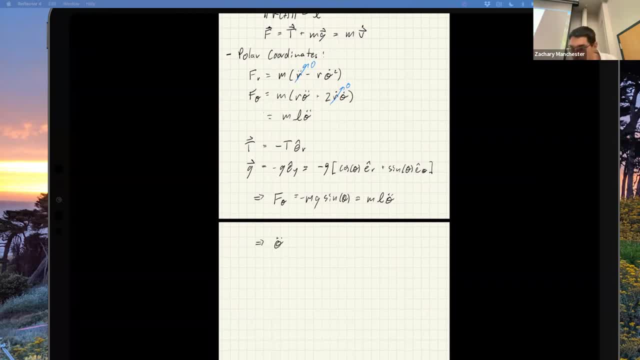 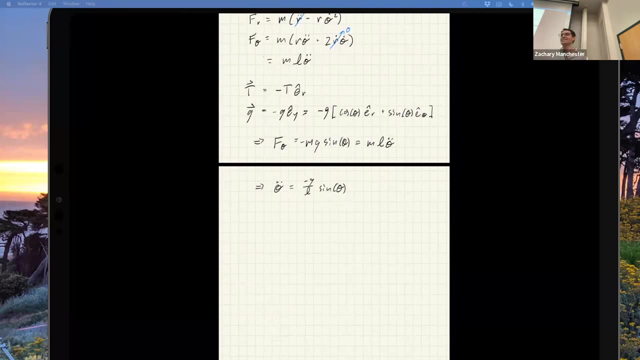 And so then at the end I get the famous thing we all know and love. OK, so that was actually a kind of gnarly application of f equals ma. right, We had to go through all this gymnastics to get these coordinate transformations to write down. 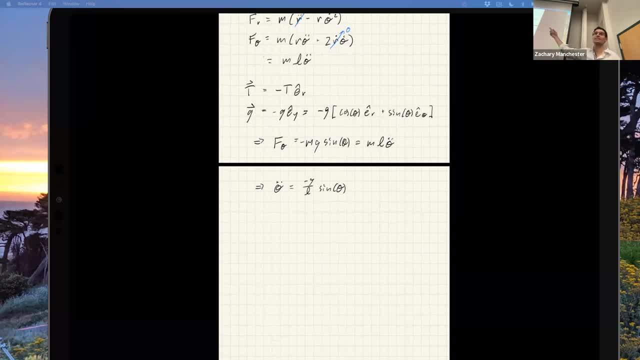 even just write down: f equals ma and polar coordinates to get to this right. So let's write down some other bonus, if anyone knows. So, does that equation have a closed form solution? It's another fun bonus question. What do you guys think? 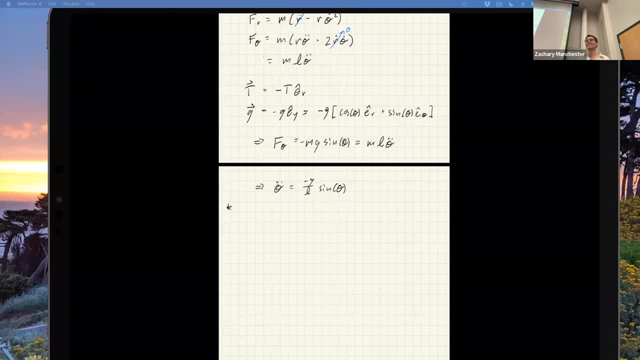 Any of you have opinions? What do you think It turns out? it does, And I'm not talking about the linearized, simple harmonic oscillator thing. This has an exact analytic solution that almost no one knows about. Just super fun. It's a very 19th century weird thing. 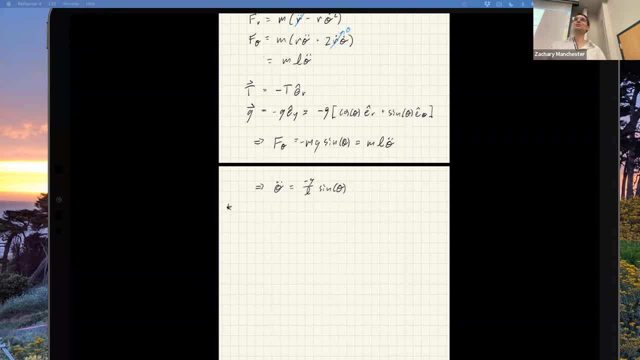 that no one cares about anymore. Turns out that has a closed form solution in terms of these things called Jacobi elliptic functions. Anyone heard of those? They show up. I've done a few weird applications But yeah, it turns out the nonlinear pendulum. 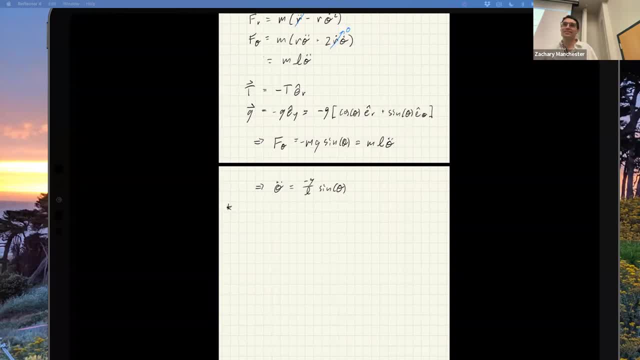 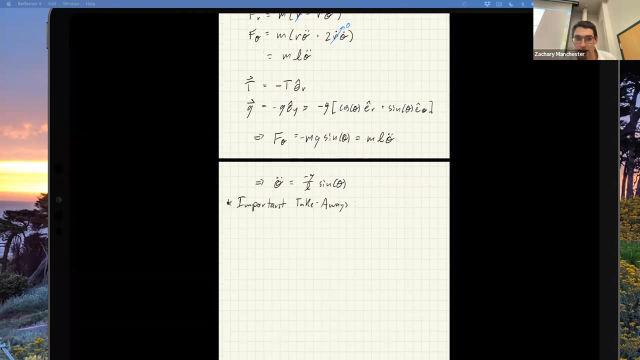 has an exact analytic solution. Fun fact In case that ever matters in your life, it probably doesn't. OK. some more takeaways, though, just to sort of let's see So the constraint there that we had to think about right. 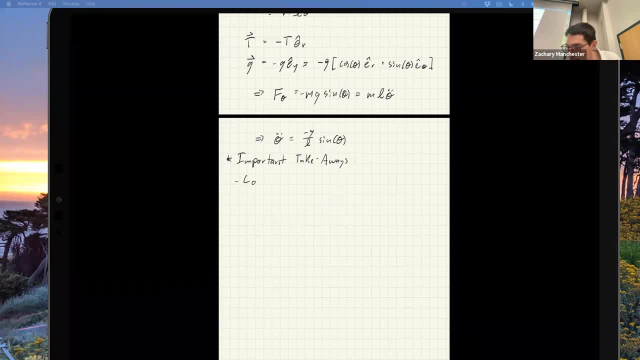 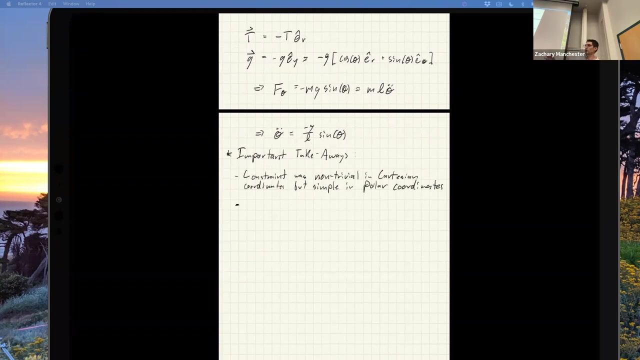 The fact that the length of the pendulum was fixed. That's a non-trivial thing to write down in Cartesian coordinates, right, It's a non-linear constraint, But it becomes super simple, trivial in polar coordinates. Let's see Basically, what happens is in polar coordinates. 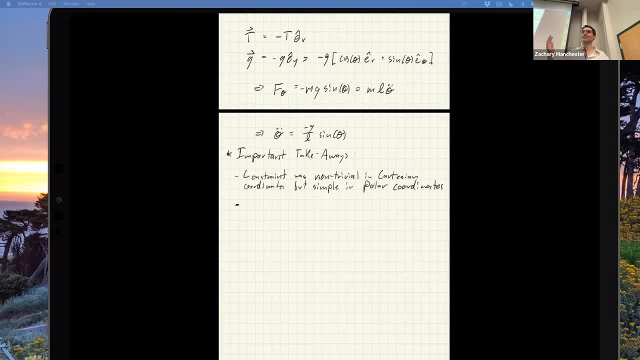 the constraint lines up with one of our coordinates. right, That's kind of magic, And then we can basically just ignore that coordinate. Let's see. the other thing that happened is we also never had to explicitly calculate that tension force. OK, 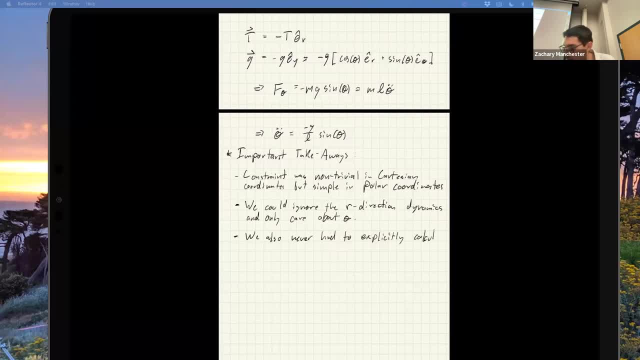 We can use a little bit of our, which is sort of cable tension or constraint force. Let's see Other things. So yeah, kind of the gain here. what hopefully should be coming apparent here is that coordinates are like a huge deal and can make your life way easier or way. 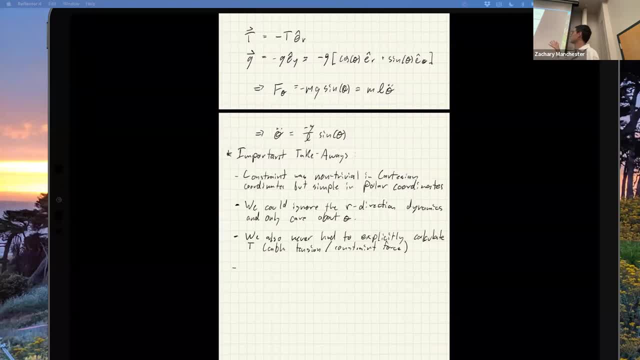 way harder And in particular, f equals ma doesn't make your life easy when wanting to specify weirdo coordinates. So this is kind of one of the reasons the Lagrangian or the Lagrangian step is so powerful and popular is that you can pick your coordinates such that basically all the 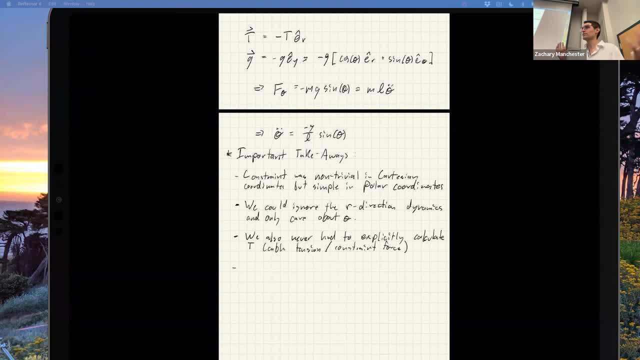 constraints drop out along different coordinates that you can then ignore, right. So that's kind of the game which you can't do in f equals ma land, right. In f equals ma land, we have to go through this gymnastics to just get to ma in a particular coordinate frame and then write. 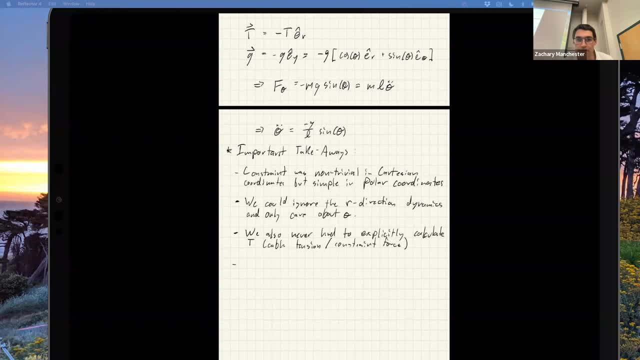 everything down and then cancel out the unneeded coordinates, right? So let's see what else is there. So this system really has one degree of freedom, which is just the theta which we all know. If we want to do it in Cartesian coordinates, then we've got to write it down as x, y and then 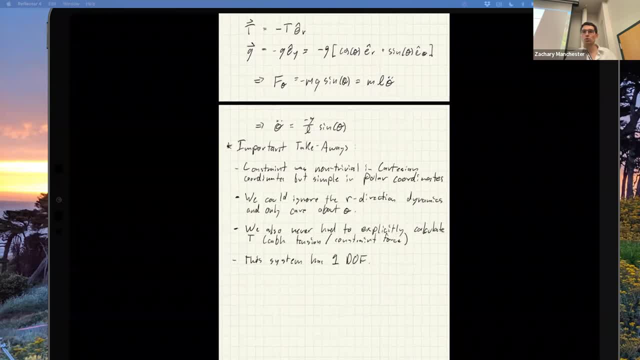 the constraint right. So if we want to do it in Cartesian coordinates, then we've got to write it down as x, y and then the constraint right. So if we want to do it in Cartesian coordinates, then we've got to write it down as x, y and then. 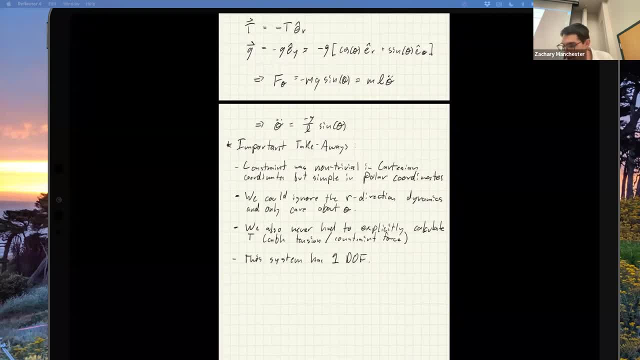 if we can write it down in terms of just one coordinate, ie theta. in this case we call that minimal coordinates or joint coordinates in robotics, sometimes So minimal because it's just enough coordinates to capture your degrees of freedom, right? So minimal coordinates means you. 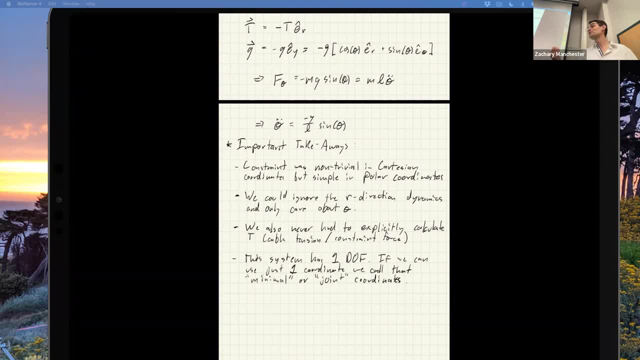 have the same number of coordinates as your degrees of freedom, It turns out that's not always a good idea in general, and we'll get to why. But if you have the same number of coordinates as your degrees of freedom, it turns out that's not always a good idea in general, and we'll get to why. 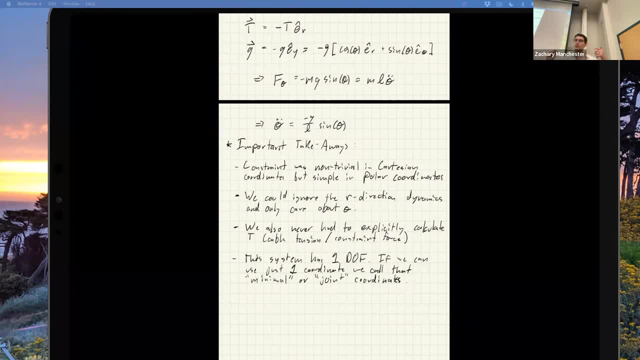 Then it's called joint coordinates in robotics, because it classically corresponds to the joint angles on a manipulator arm as your minimal coordinate set for something like a robot arm. You'll also hear the term generalized coordinates, which is more of a physics term, which is actually 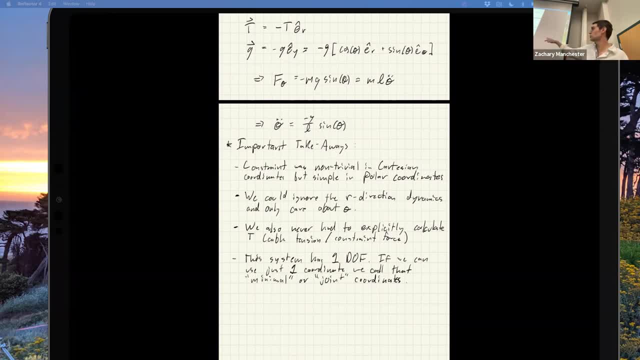 often used synonymously with minimal coordinates, but isn't actually the same thing. You can have generalized coordinates that are not minimal, So we won't do that. And then the sort of comments on this I'd say most current, like state-of-the-art robotic simulators, use minimal or joint coordinates. 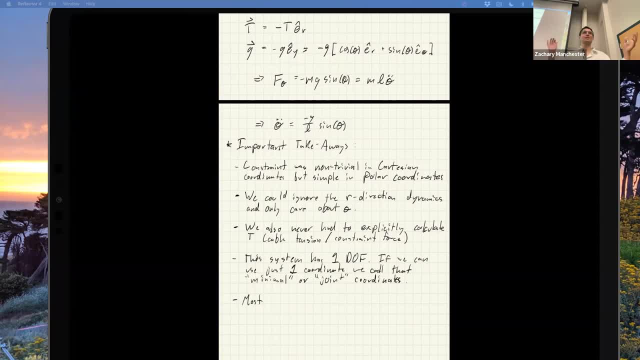 So this is sort of why you've seen, you know Q's and Lagrangians your whole life. It's because this is kind of a standard thing and this is what most current simulators do And you might think sort of, you know, that's a good thing. You want to use the least number of variables possible and have the most compact, like state vector or whatever. 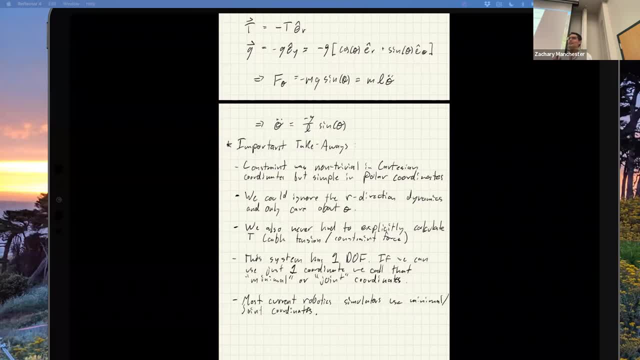 Turns out that's not always a good idea and it's not even always computationally cheaper to have a smaller state. Okay, But intuitively that seems like a good idea, right, Which is kind of maybe why all the current stuff does it this way. 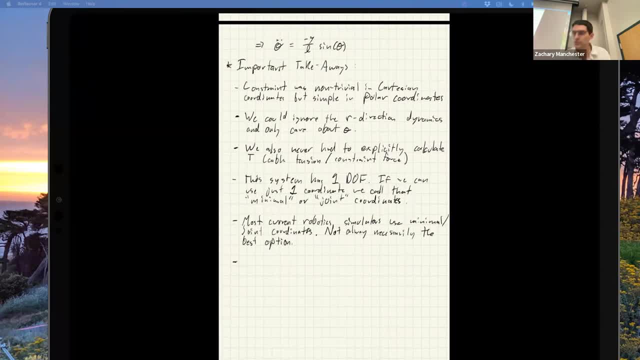 Okay. So there is sort of this opposite extreme where we could, in this case, like write down the full Cartesian position of everything right And then write down constraints, So in this case the unit norm or the length L constraint right for the pendulum. 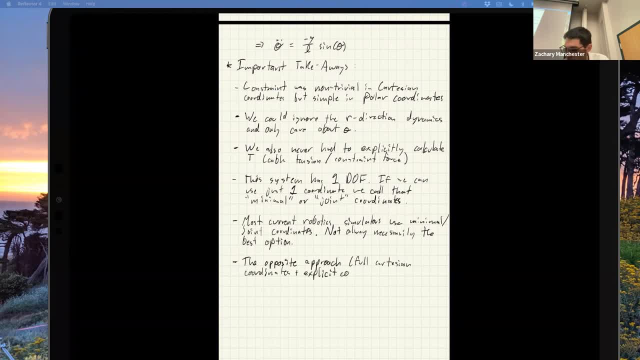 And then write down explicit constraints. This is often called maximal coordinates, And less popular, for not particularly good reasons turns out, But there have been, you know, situations where this is a good idea. I kind of like this, And we'll do more of it.